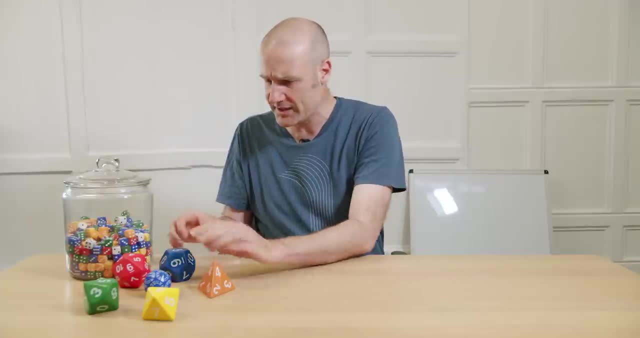 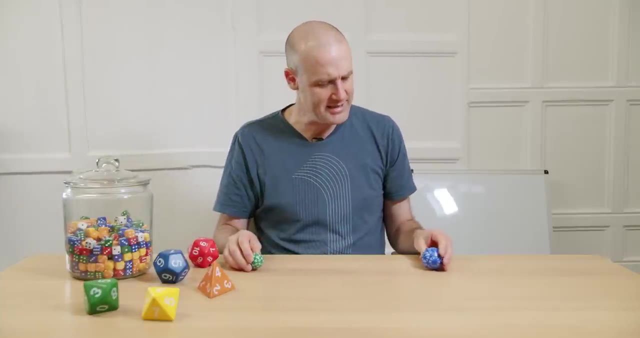 I've got like the D4, so D for dice and then 4 for 4 sides, D12, D20, classic. I mean. just for overkill, I've also got my D60 and D120, which is completely unnecessary. 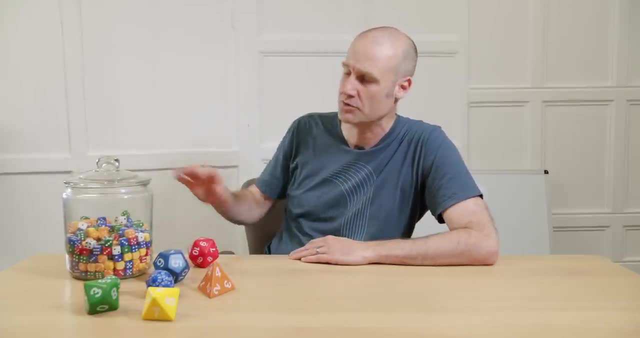 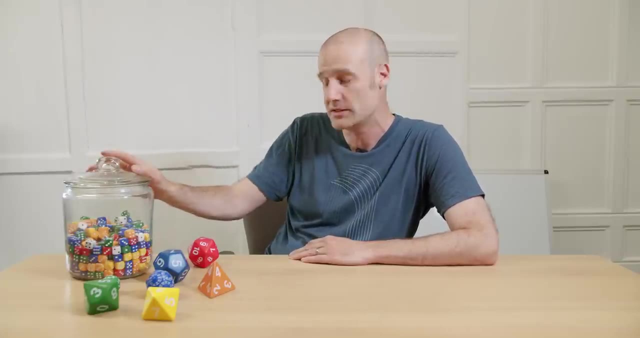 And, of course, the staple of the dice world, a candy jar's worth of D6s. Anyone who visits me in the office can just grab a couple of these as a treat, And so Gilad's question was not actually about the numbers or the geometry or anything on this dice. 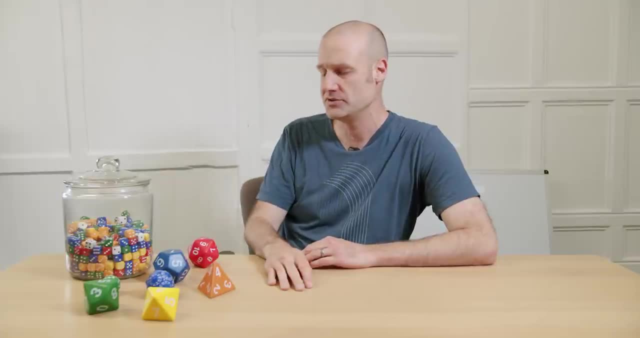 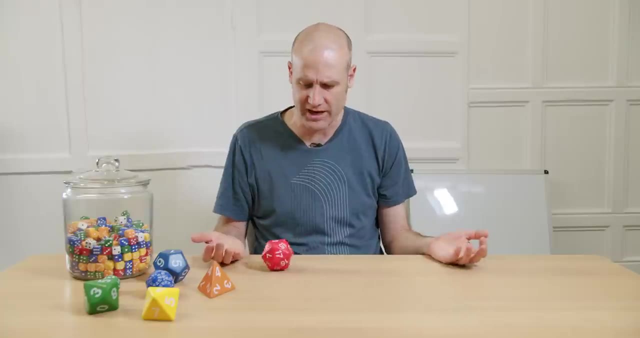 It's about a modification you can make to Dungeons and Dragons. So if you're rolling a D20 for some reason like you need a high number, so something good happens to your character. So I just roll, let's roll 12.. Not bad. 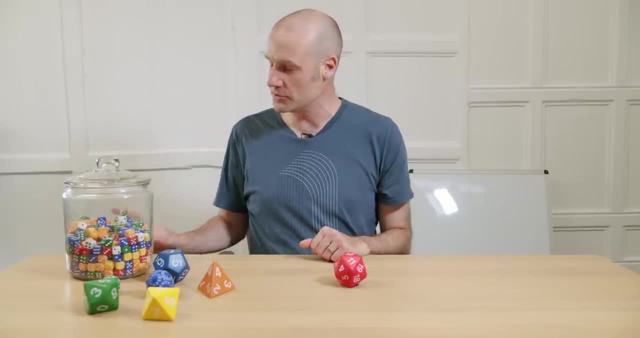 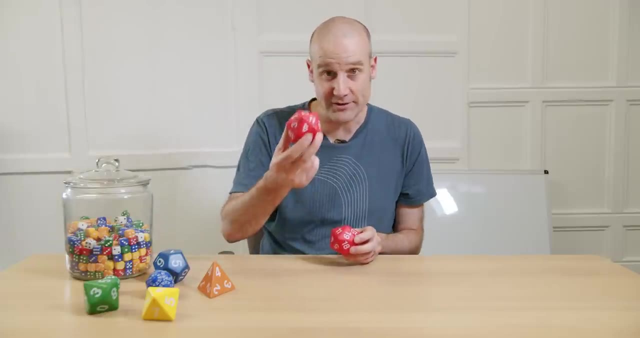 But what if you want to give that player an advantage? What you can do is bring in a second identical dice. So instead of rolling just the one dice, you roll one dice and a second phantom dice. So on the main dice I've got 11, and on the phantom dice I've got 4.. 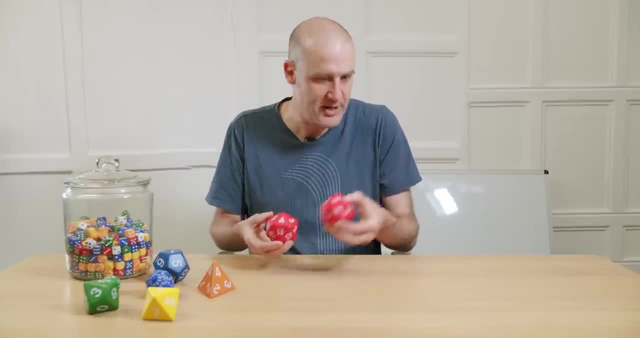 Okay, at that point you can choose whichever one you want. So you pick the better one, the higher one, So you go, I rolled an 11.. So every time you roll, if you have with advantage, you roll two dice. pick your favorite. 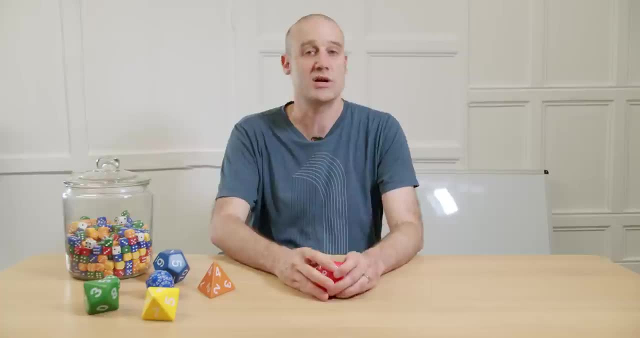 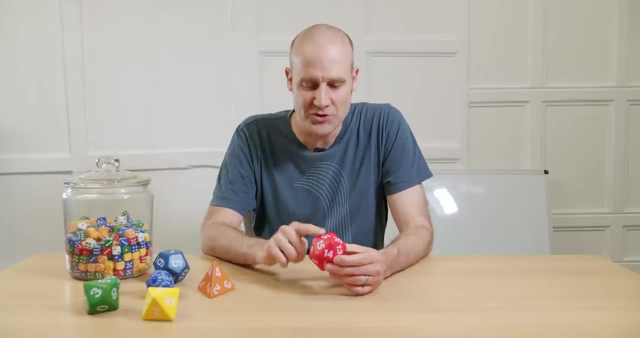 in this case the 16, and discard the other one. And Gilad's question was: if you're rolling two dice, picking the best one, so you have an advantage. what is the new average value? What is the expected value from rolling identical dice at the same time? 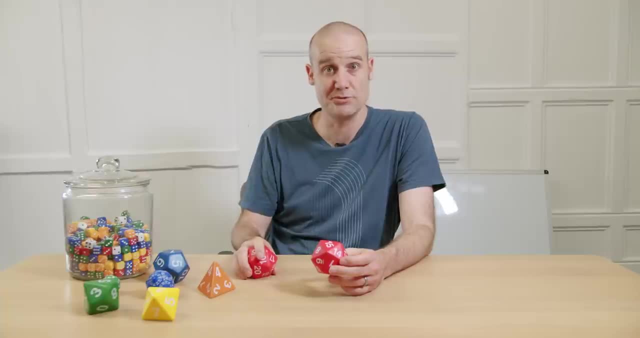 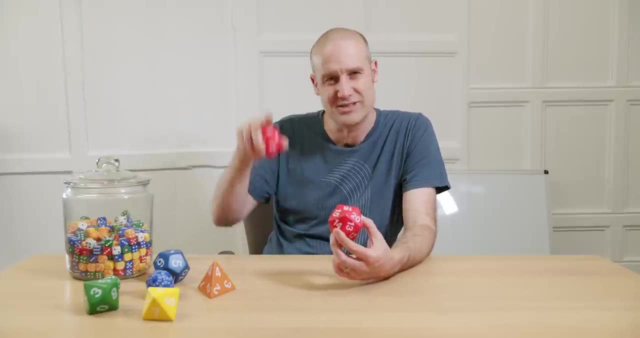 They did look online first, which I appreciate people doing that before they email me. But all I could find was people putting values into spreadsheets, like on a case by case basis, and then taking the average manually. And don't get me wrong, big fan of spreadsheets. 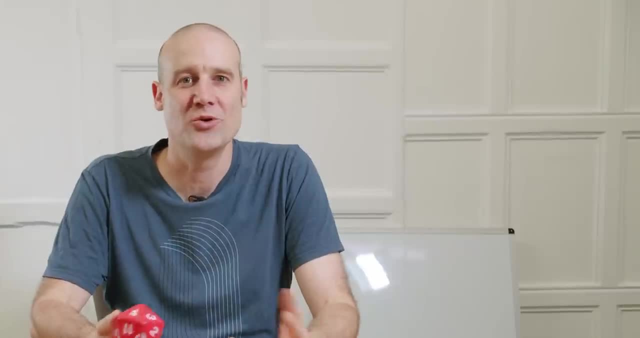 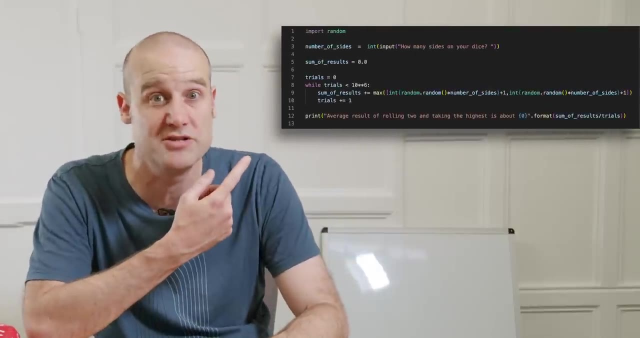 But we can do better. My zeroth step, as always, was just to simulate it in software, So I put together some terrible Python code. This is it here. It's not great. I'll link to it below if you want to check it out. 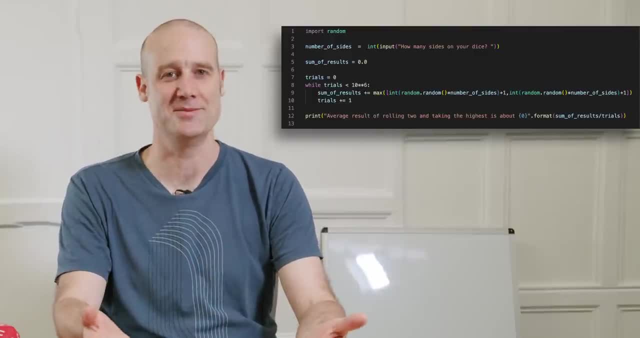 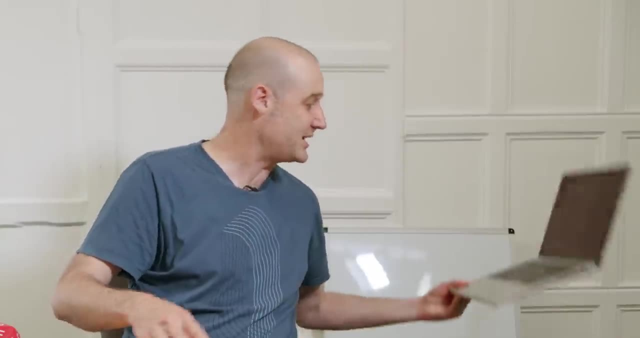 It just rolls two dice a million times, keeps track of which was the maximum value, adds them up and gives you the average at the end, And I've got my laptop here running that exact code, which you can now see next to me here. 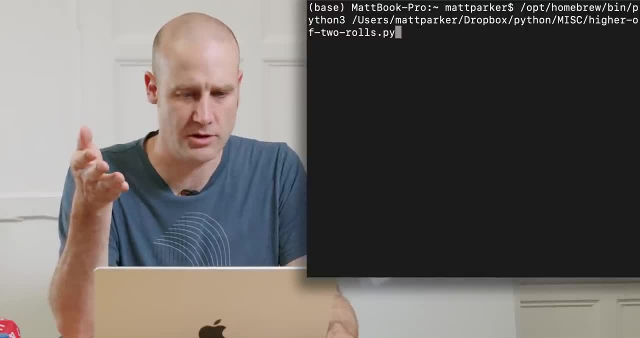 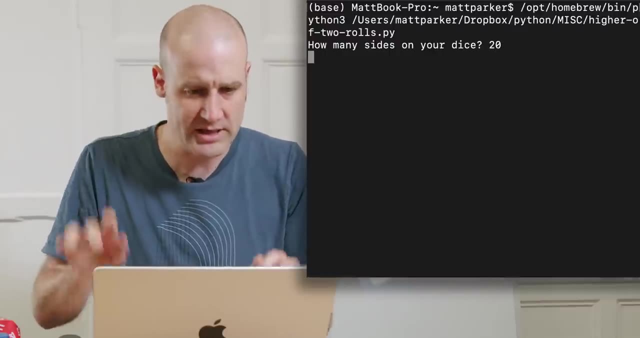 So this line that's just saying: run some Python code that I've called higher of two rolls, And if we run that it asks you how many sides on your dice. Let's do the d20.. Doing a million rolls and there it is. 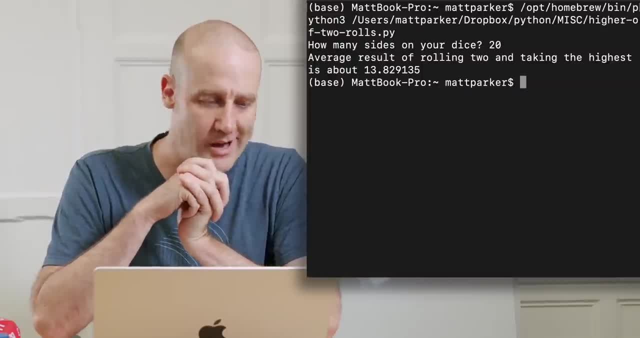 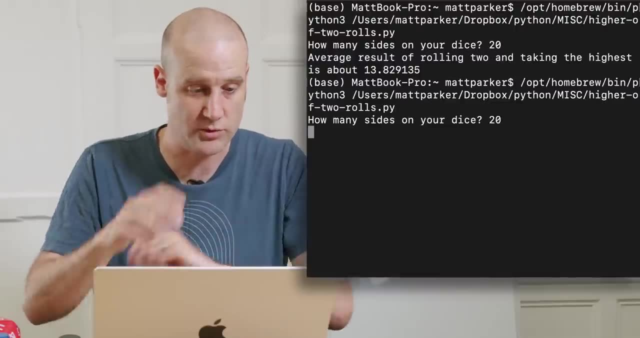 The average result of rolling two and taking the highest is about 13.829.. You think was that accurate? Doing it a million times, We can redo the same thing again. Let's do another 20.. This time 13.83.. 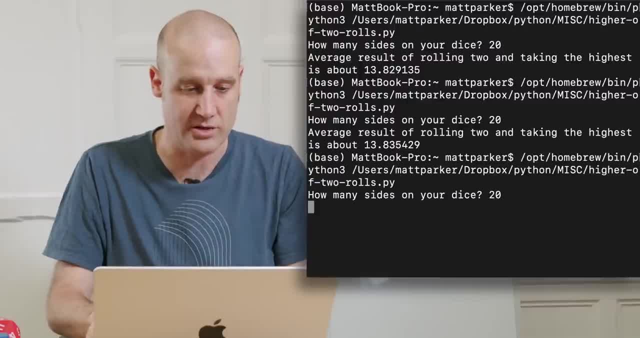 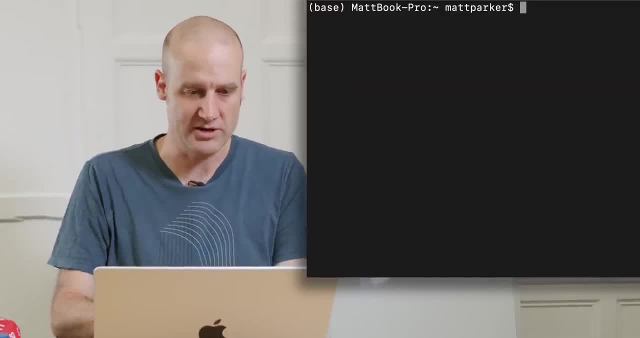 Okay, so we're always getting about 13.83 for 20, give or take, So we can be reasonably confident. that's roughly the right value And, of course, let me clear that You can do that. We did that. four: 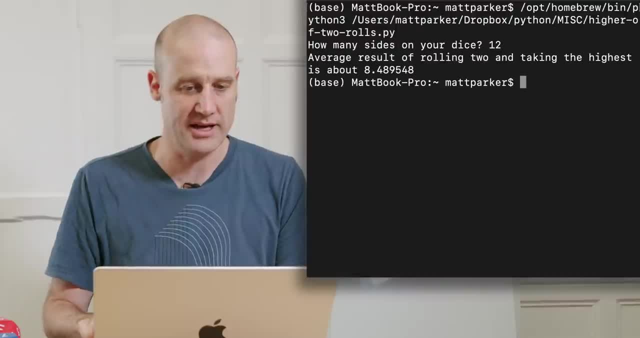 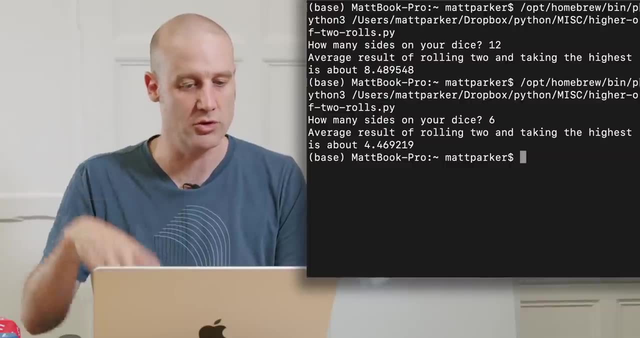 Let's do the d12. Then you're going to get an average of about eight and a half. We try it for our friends, the d6 over here. It's going to be around about 4.47-ish. So now we can get these results. 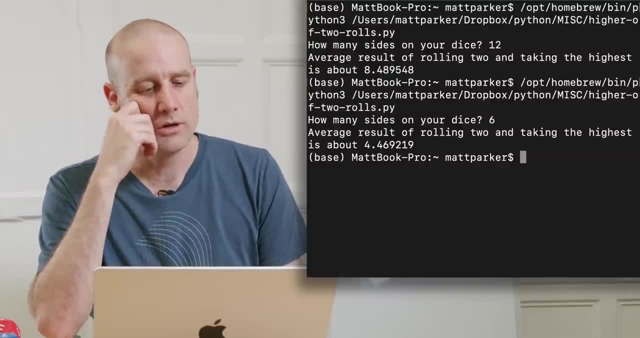 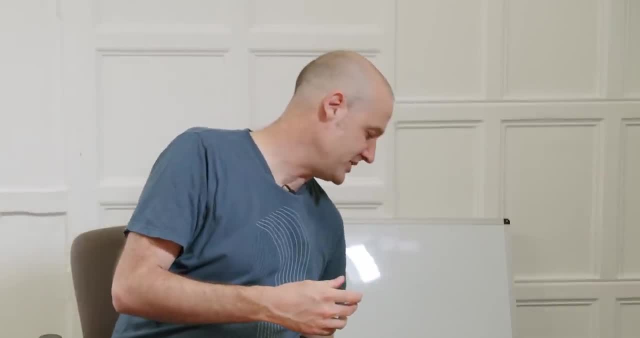 and we're confident they're correct. Now we have to crack the logic behind it With some tweaks to the code. instead of just getting the average value, you can, of course, get to spit out the probability of getting any given value, And this is what Gillad did. 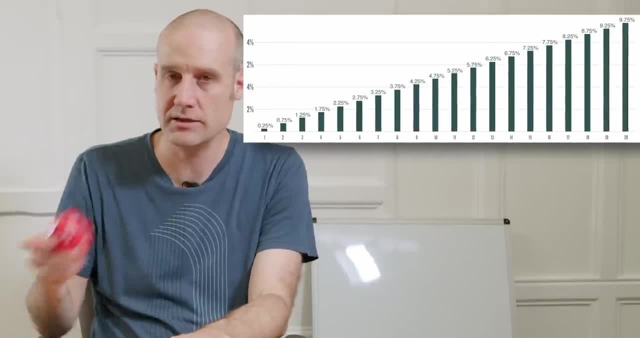 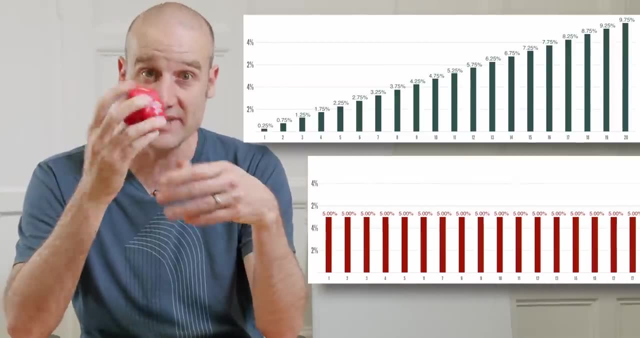 and they did a plot For the record: a single d20, every single face has a one in 20 chance of coming up. That means they're 5% each, And if we did the chart for this, it would be a bar chart where every single number is 5%. 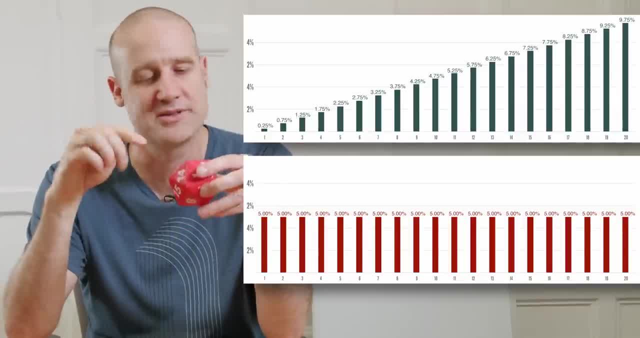 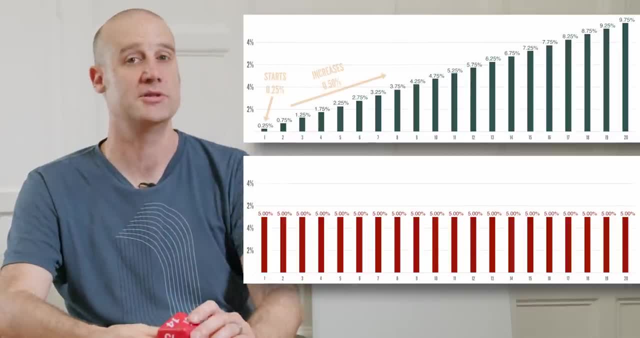 Perfectly flat And I've not joined it together as a line because it doesn't make sense to have an in-between value. I've just done a bar for every single value to show you the percentage, and what Gillad had plotted was the same thing. 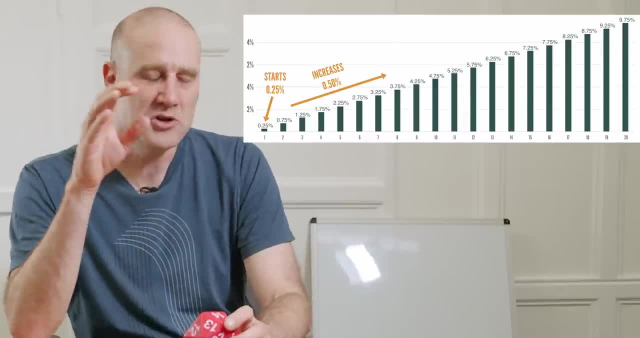 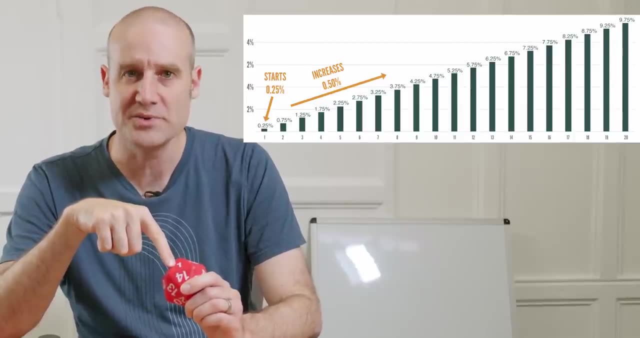 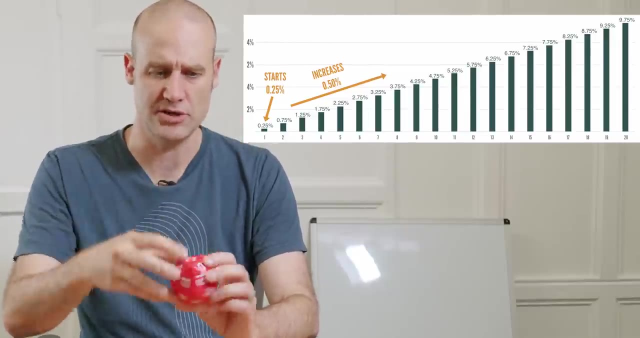 but with rolling for advantage And you can see you get a perfectly straight line. It starts with a 0.25% chance of getting a one and then it goes up half a percentage point. every single number you go up on the dice. 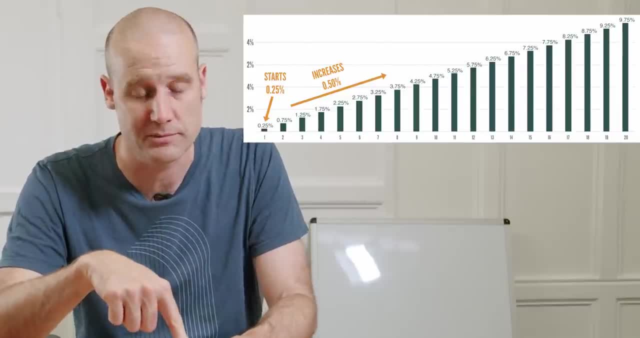 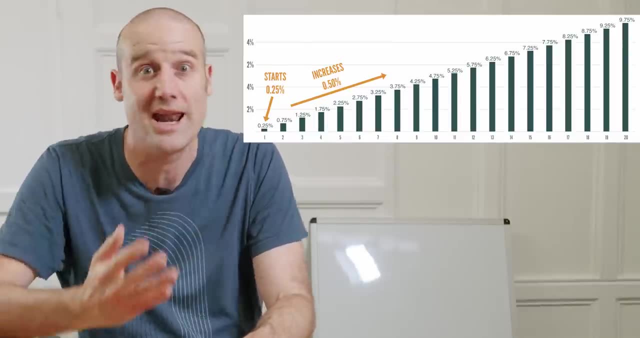 until 20, which is the most likely, is the biggest is a 9.75% chance. And we're like that's interesting And we'd run the simulation over and over and we'd check the numbers and they add up to one. 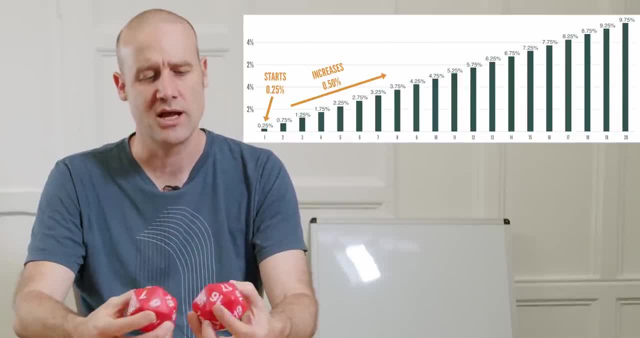 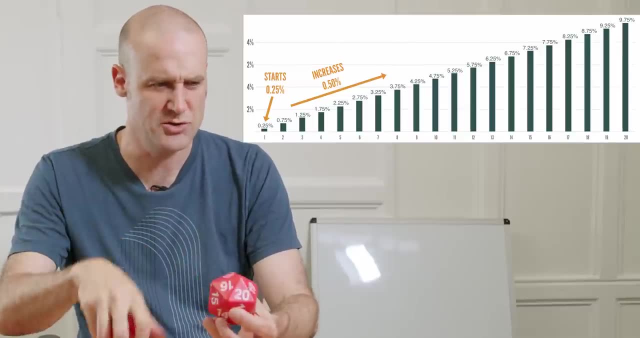 so the whole thing holds together. So now we had two questions. One was why, when you plot the probability for each of the different faces with advantage, do you get this perfectly straight? arrangement of the probabilities And secondly, the average. 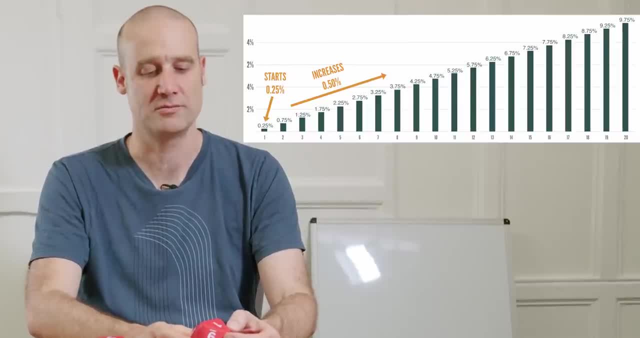 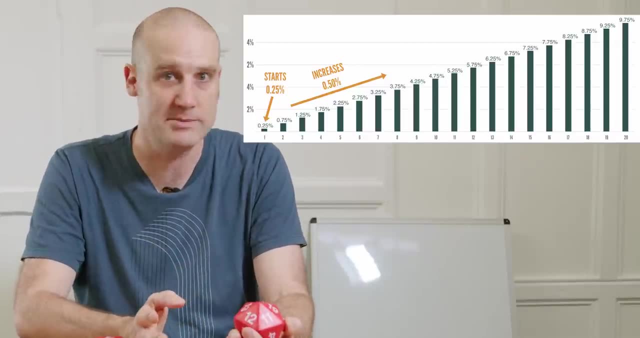 Gillad noticed is always about two thirds Of the maximum value. I say about two thirds it's going to be some weird number, probably involving E. It won't be that simple, But they had spotted roughly two thirds and we had to answer both those questions. 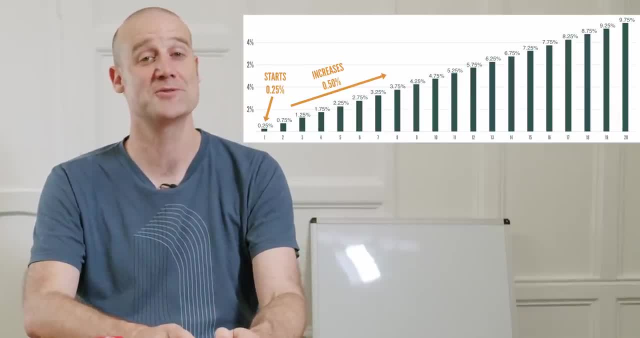 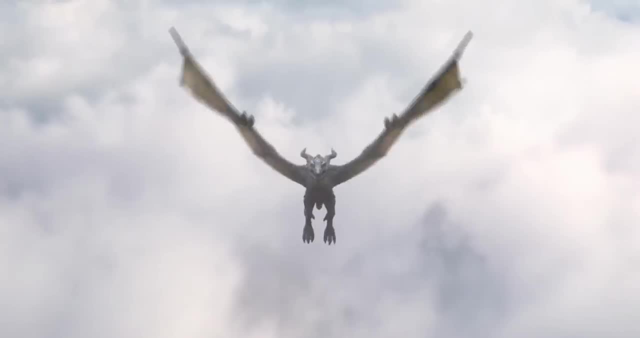 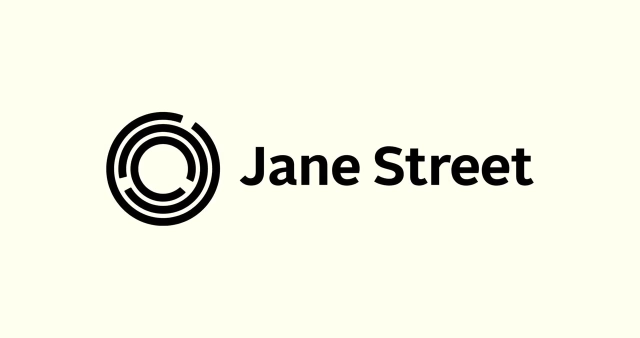 And, my goodness, I was not expecting the result we got. This video is brought to you by Jane Street, who are also supporting the 2020, the 2022 International Mathematical Olympiad. Try a sample puzzle at the end of this video. 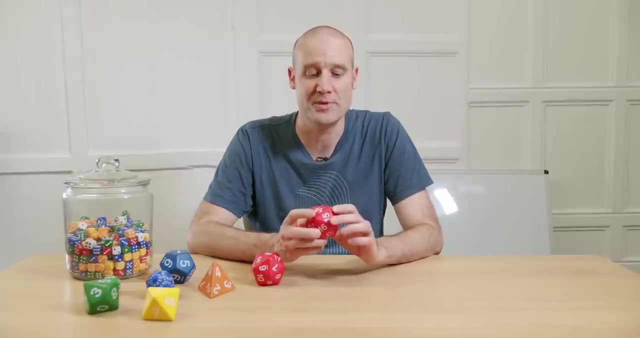 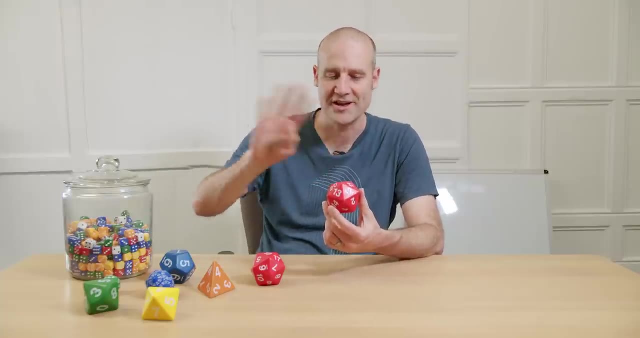 Jane Street have actually provided a brand new IMO style puzzle that you can try. We'll put it at the end of the video, but it's based on an icosahedron. not the dice, just the actual shape. Super interesting. 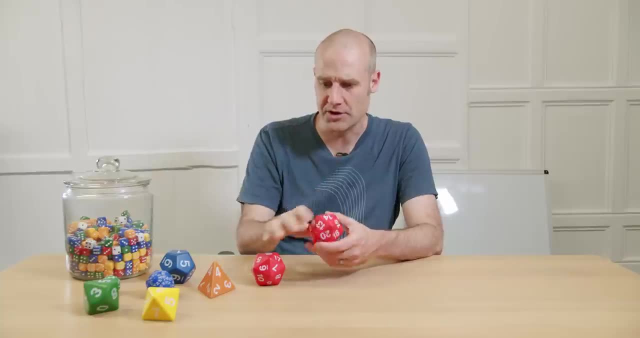 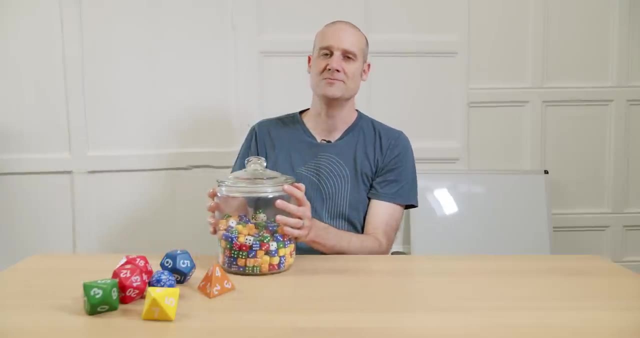 Check that out at the end, But for now we're going to try and crack what's going on with the probabilities when you roll for advantage. We're not going to do the D20, though That's a little bit too much. We're going to start with our friend. 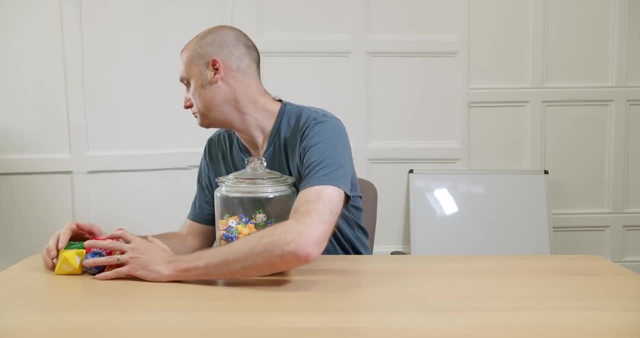 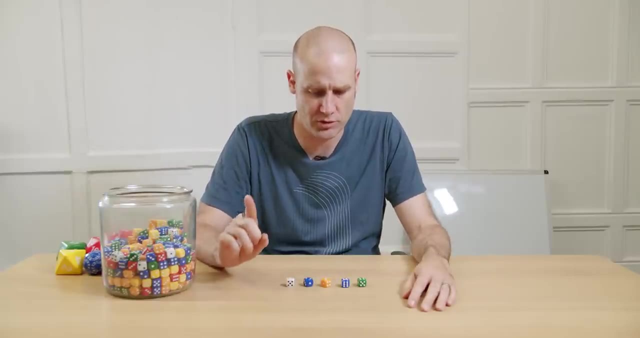 the D6.. Oops, That's gone. Here I have some D6, and we can look at what happens if you roll two distinguishable D6. So I've now got a green one and a blue one at the same time, And each of them could have. 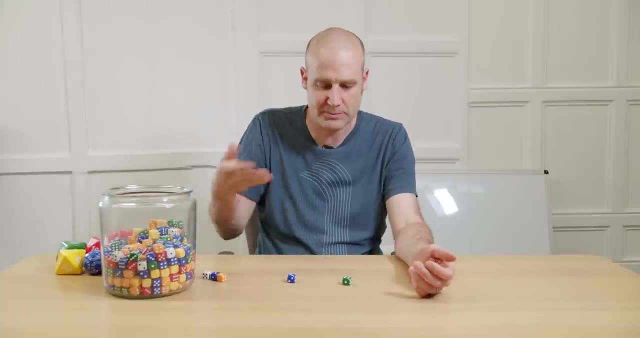 Oh, I've got two fives. There you go. Each of them could have any of six possible values: a four and a three. So we can do a two-way plot where we've got all the values the blue can have on one axis. 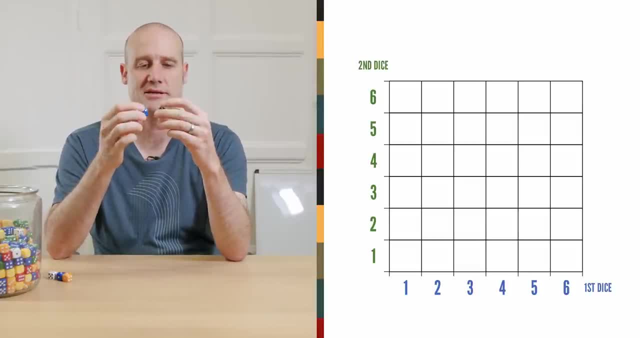 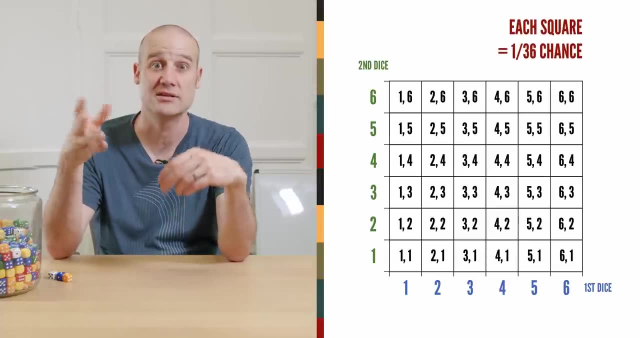 all the values the green can have on the other axis And inside each square we can have, we can put what that combination is And, importantly, each of those squares has a one in 36 chance of happening, because that's just six squared. 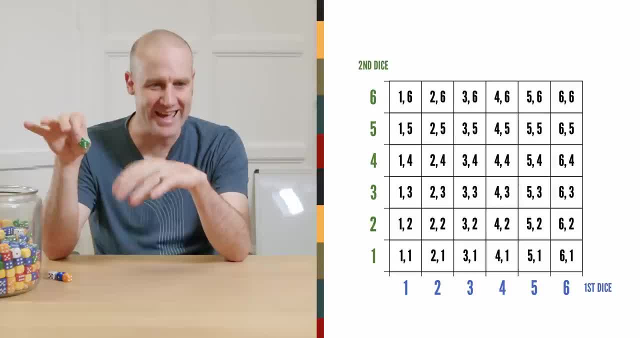 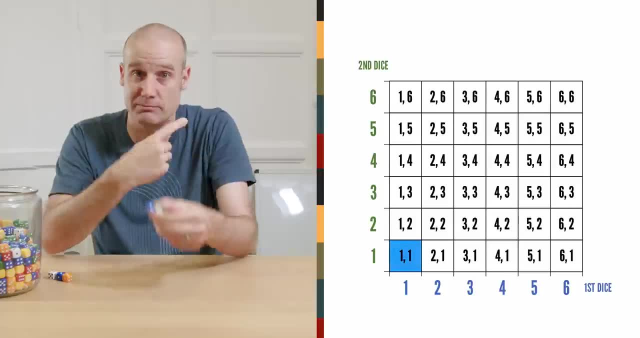 We can now go through and colour in what values we would get if we rolled that pair and we picked the highest. So the only way to get one is the bottom corner. So there's a one in 36 chance of doing that. There are three ways you can get two. 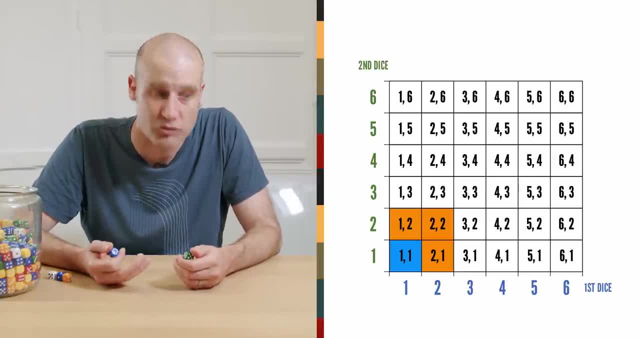 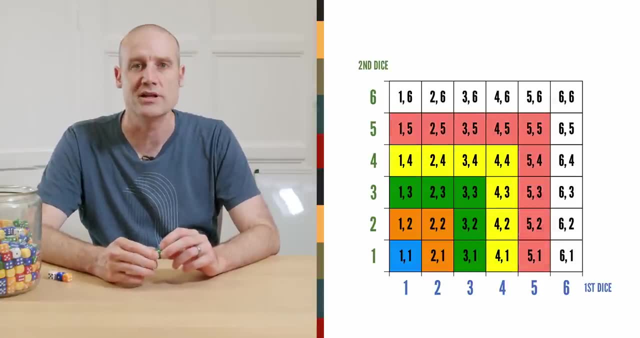 If you get any of these, you would choose two as the biggest number, So that's a three out of 36 chance. Here's all the ways you could get three, and then four, and then five and finally six. And then I realised what I was looking at. 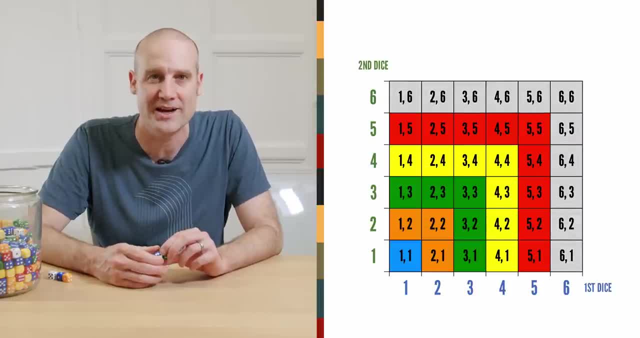 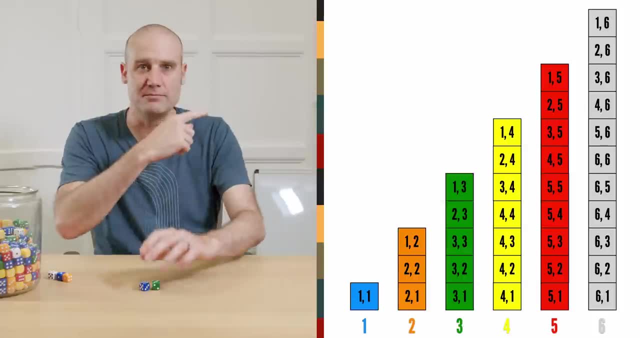 is the same bar chart from before. In fact, we can just stand these up And there you are. That's our bar chart, because the probabilities are proportional to the number of squares And that's why you get that straight line. It's because, if you add, 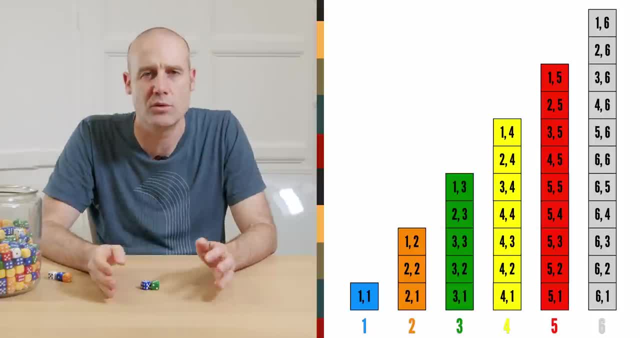 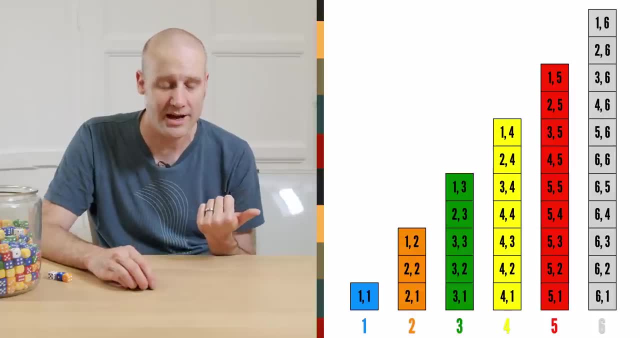 consecutive odd numbers: one, three, five, seven and so on, you get the square numbers one, four, nine and up, in this case 36.. And I was so excited when I realised this, And so we can see the numbers. 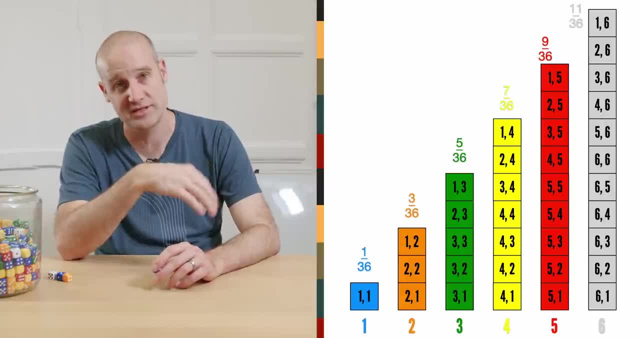 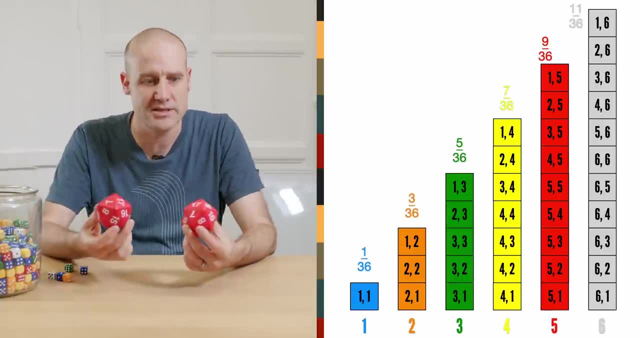 for the case of the D6, because it's one over 36,, three over 36,, five over 36, and so on. 36 is just the number of faces squared. So if we want to go back to our D20s, 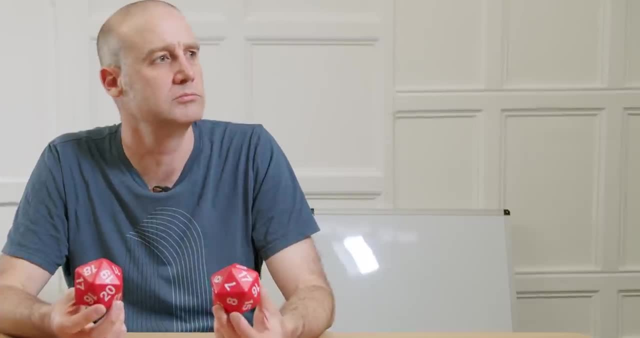 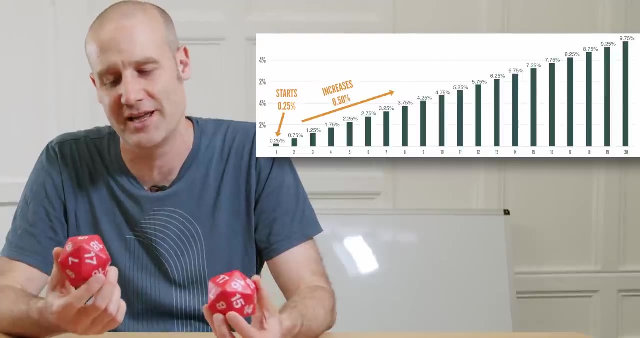 it's just one over 20 squared, Wow, One over 400.. That's 0.25%, which is why we had 0.25% likelihood for getting a one if you roll with advantage, And then it goes up by double that. 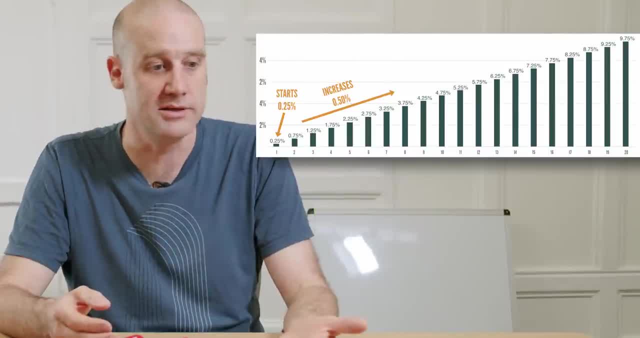 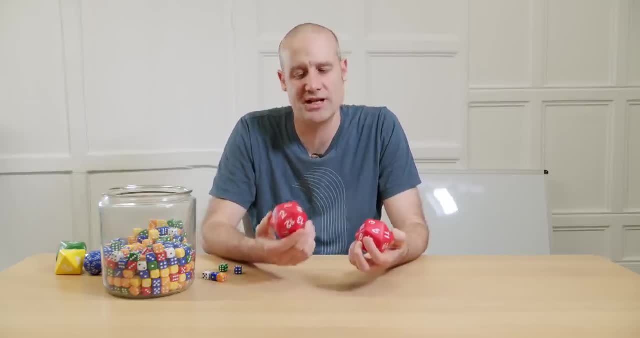 every single time. So the next one up is 0.75%, all the way up to 9.75%. That's where the straight line comes from. I'm so pleased when you start with a probability question and then you can turn it. 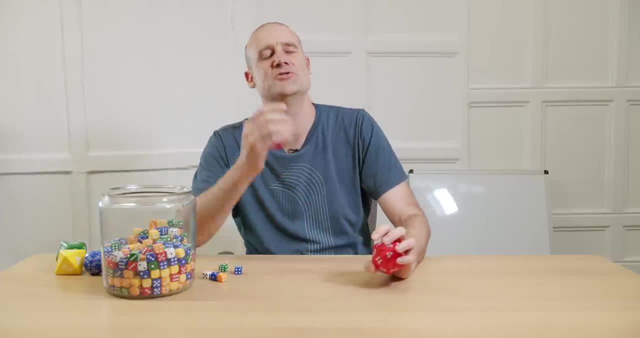 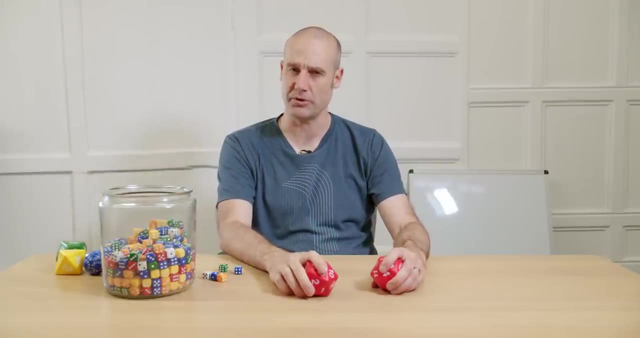 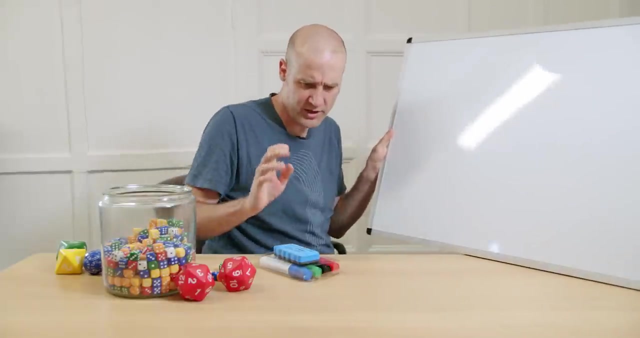 into a geometry question. that then gives you your probability bar chart for free. Ah, so pleasing, But now where does the average come from? It's working it out time, So we're going to do this in general for an n-sided dice. 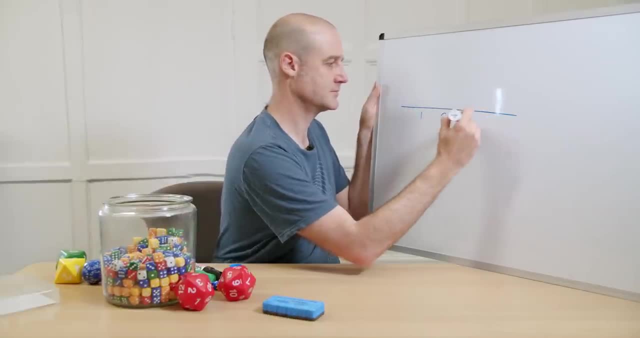 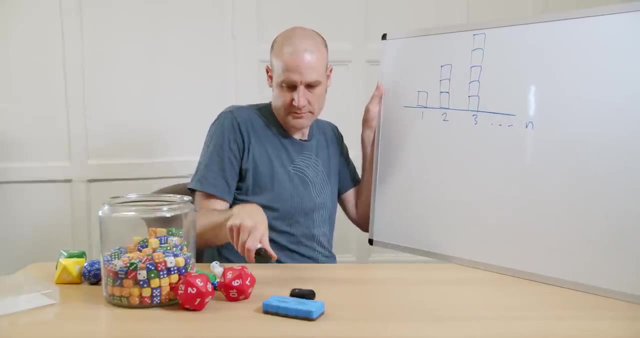 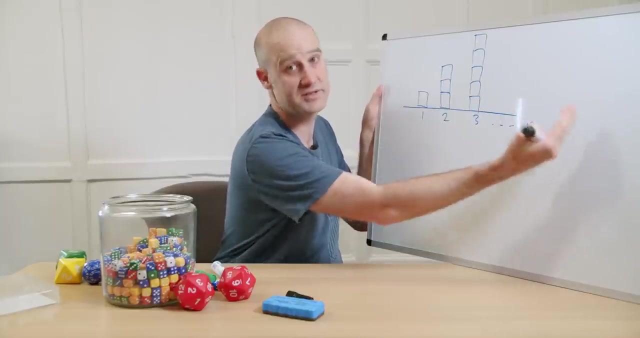 Bear with me. Okay, so we don't know how many sides the dice has. We got n sides, but we know it's going to be like this: It's going to get two higher every single time until you get to n Each of these. 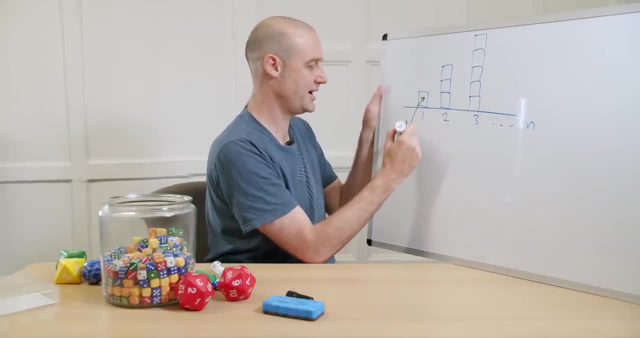 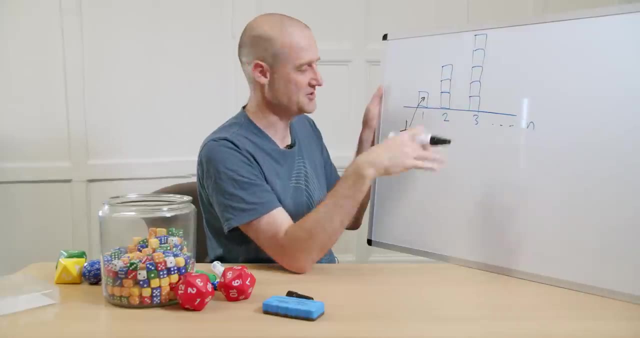 represents a probability of one over n squared, Because we know there's a total of n squared of these n, Because if you collapse them all back down again, you get your square, So good. The question now is: for each of these values on the dice, 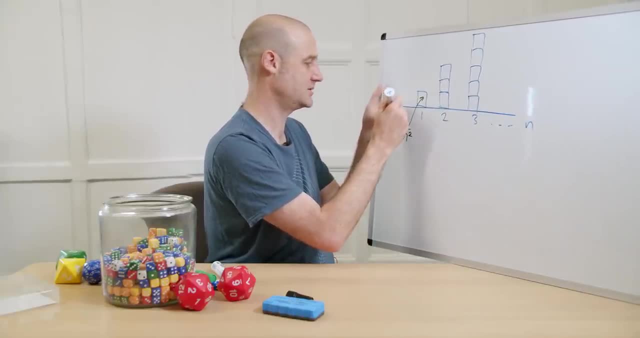 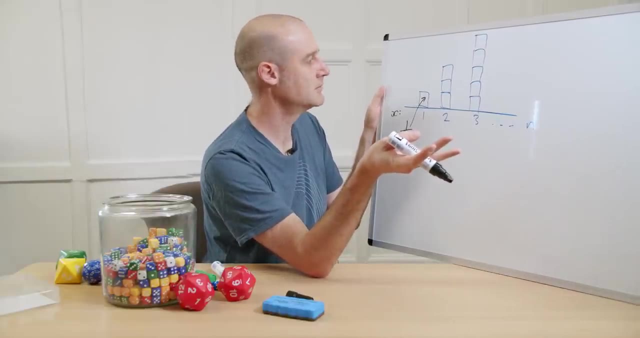 which I'm going to call these x, just because we've already used n. how do we know how many blocks are above them? Well, these are just the odd numbers. So that's 2x. Ah, let's go minus one. 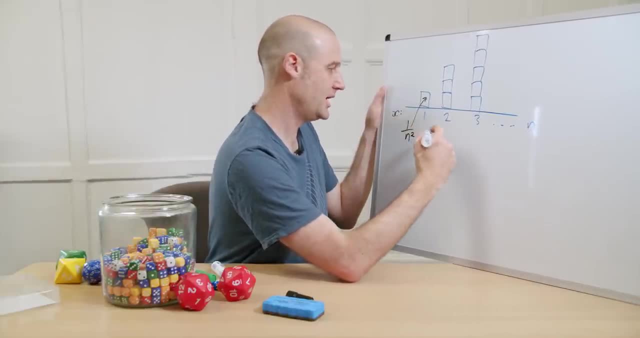 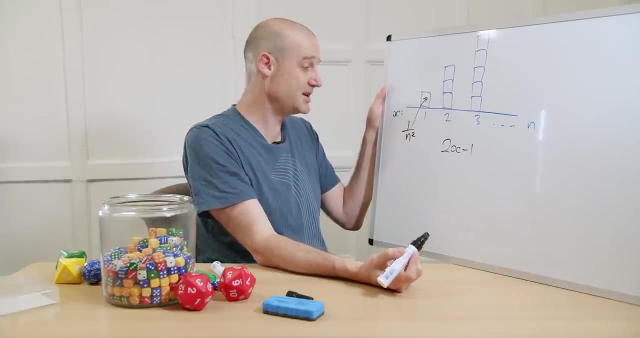 So it starts at the right point. So we know each of these has 2 times x minus 1 plus 1.. x minus 1 blocks above them, And the probability is then that times 1 over n squared. So I'm going to put that. 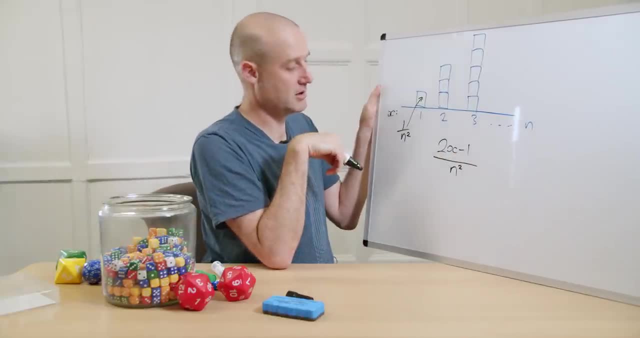 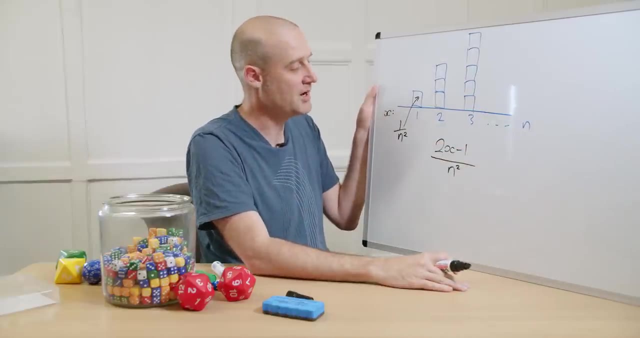 on n squared. So there you go. So for any value, x on an n-sided dice, this is the probability of getting that if you roll two of them with advantage. So what's the average value? Well, it's the chance of getting a value. 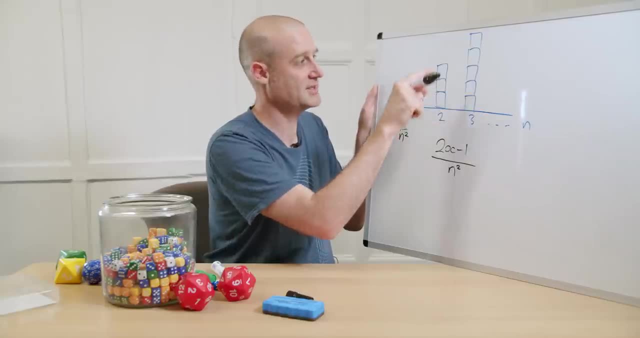 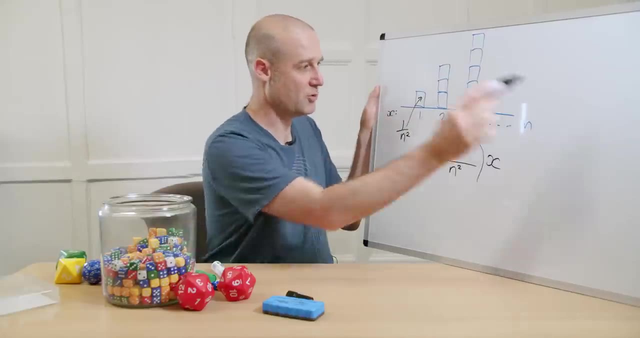 of 1 times 1.. Chance of getting 2 times 2.. Chance of getting 3 times 3.. This is the chance of getting x times x times x. And then you've got to add them all up. Future Matt here. 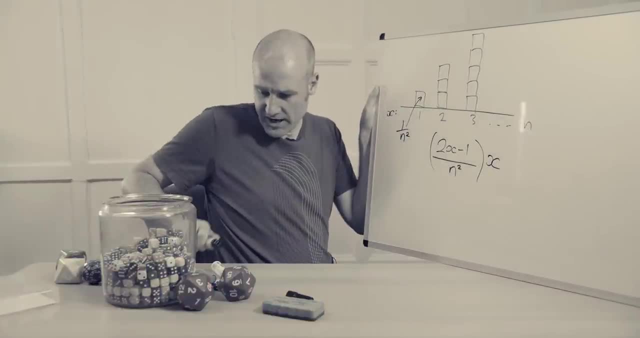 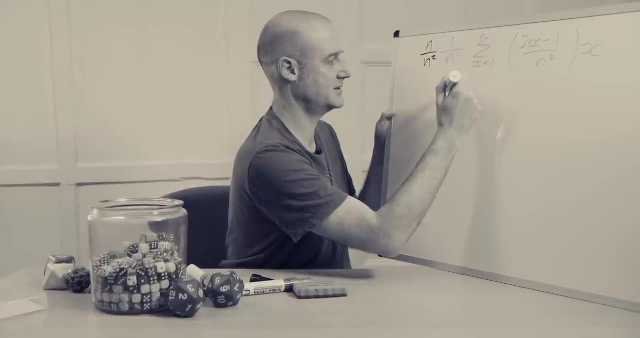 in the edit because I realised past Matt was getting a bit confused. I did have to do the summation of each of these values, The probability times the value of each face x, But I put a 1 over n at the front, which you can see there. 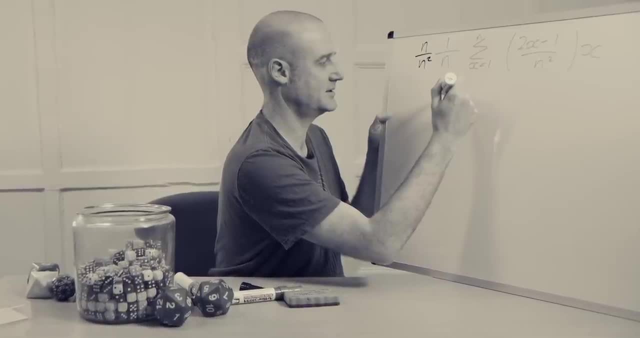 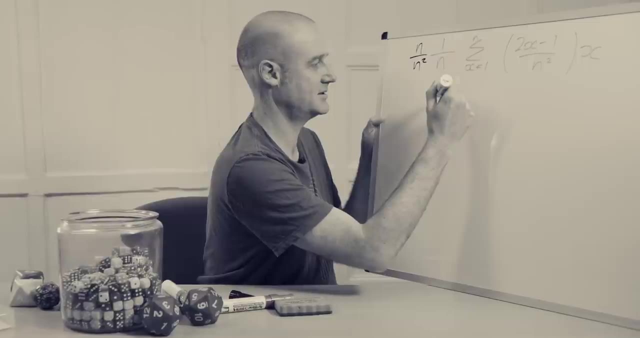 I was getting ahead to where I wanted to do the ratio And then I changed my mind. so later on you can see when I was bringing the 1 over n squared at the front, because it's independent of x in the summation, I put an n there. 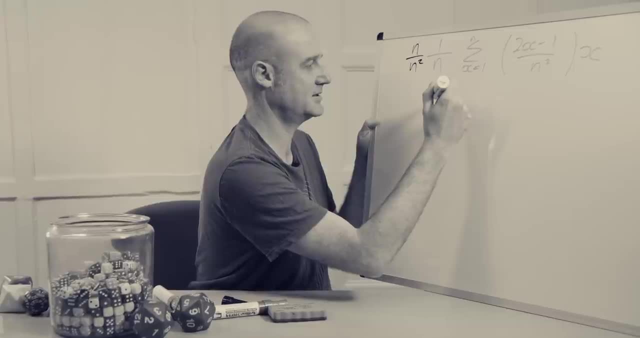 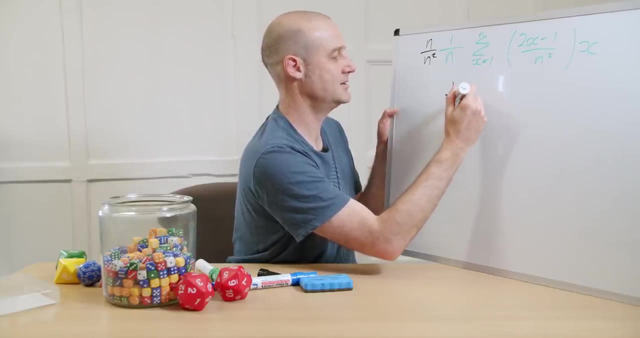 because I didn't know what I was thinking. But the point is, it all works. Don't worry about the top line, Everything is perfect from here. So it ends up being 1 over n, squared outside the sum of what we had before. 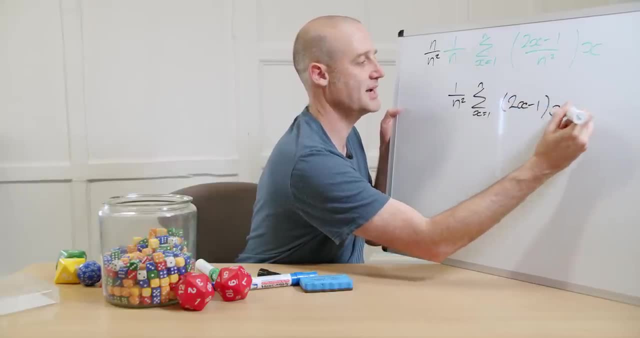 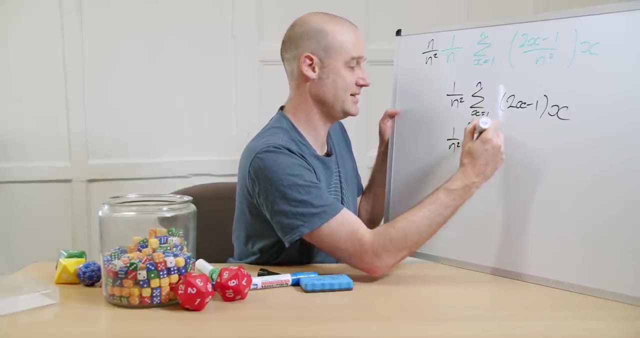 But now over here we've only got 2x minus 1 times x, And I just worked out what that was before and I remembered it: It's 1 over n squared. and then this thing: here is n on 6 times n plus 1. 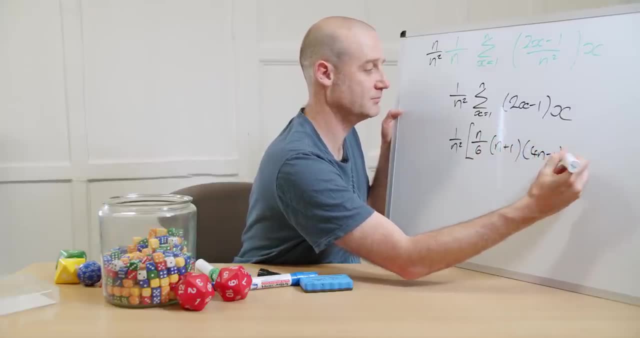 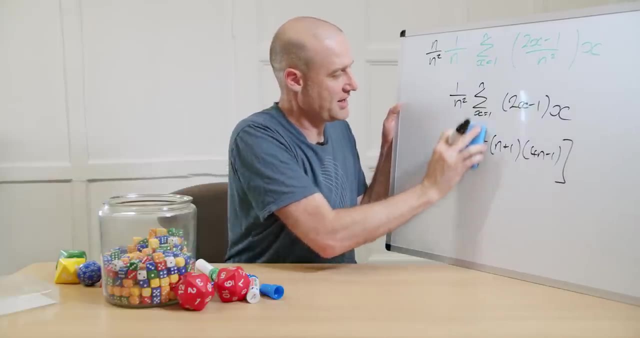 times 4 times 4.. n minus 1.. And that's it. And you're like: hang on, I can cancel this out, because if I've got an n squared there and an n there, what I've actually got out the front is just a. 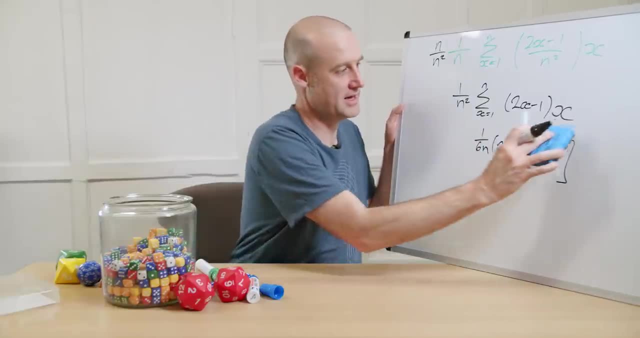 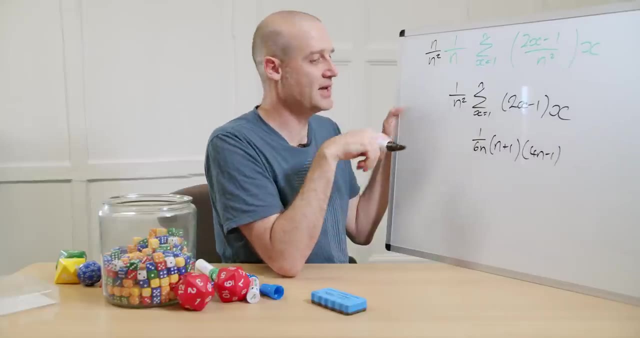 1 over 6 n, and that's it. That's our equation, And sure enough it works. If you put n equals 20 into that, you get out 13.825, exactly what we got from our simulations. If you put in n equals 6. 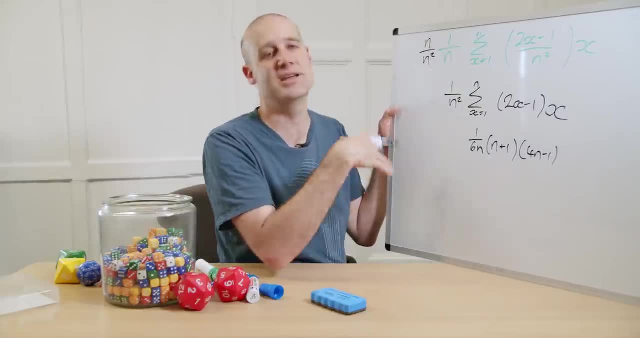 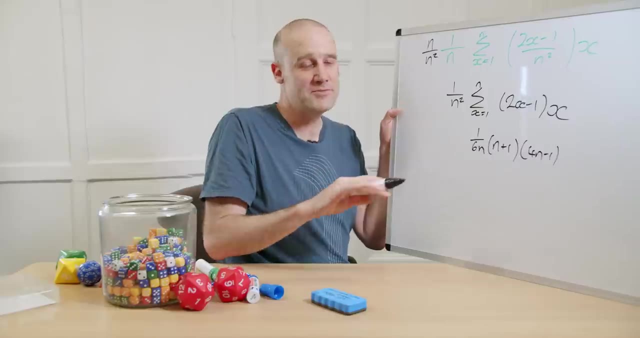 you get the same result that we got in the first result that we got from our simulations. This is the equation for the average value for any n-sided dice if you roll two of them with advantage. All we have to do now is work out where that ratio. 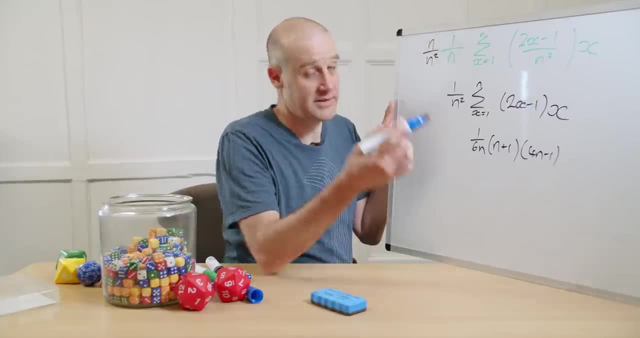 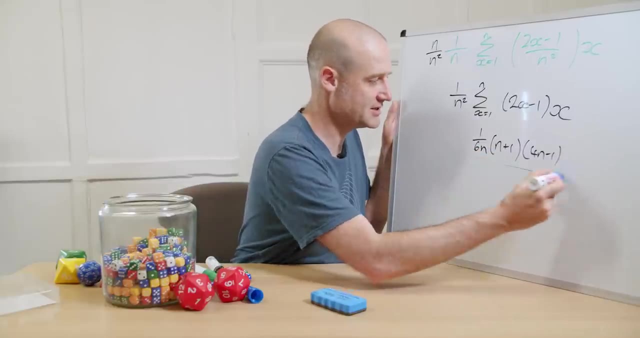 of approximately two thirds, comes from, And that's not so bad to do, because the ratio we're talking about is the ratio of this average to n. So we just got to divide this whole thing by n, which, yes, I could have just squared that n. 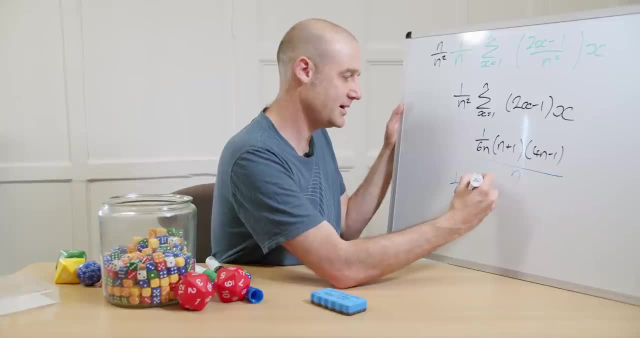 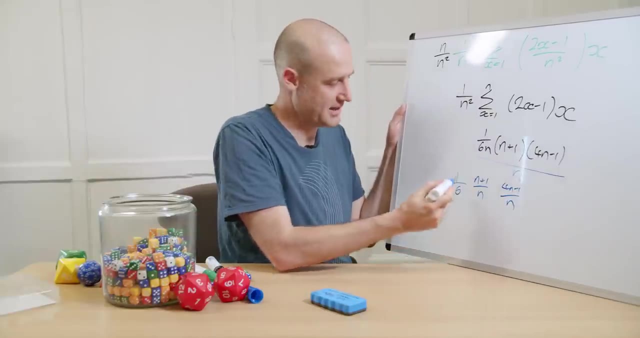 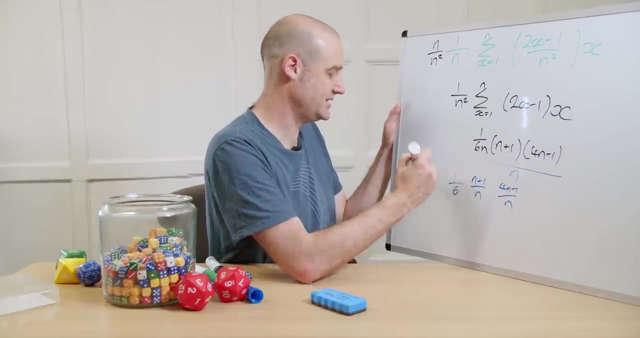 But I'm going to write that as one over six. n plus one on n, four n minus one on n. Convince yourself, that's the same. These are all multiplied together. We want to know what is the limit, as n goes to infinity. 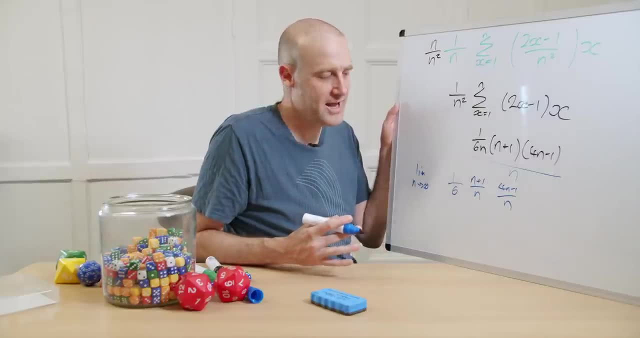 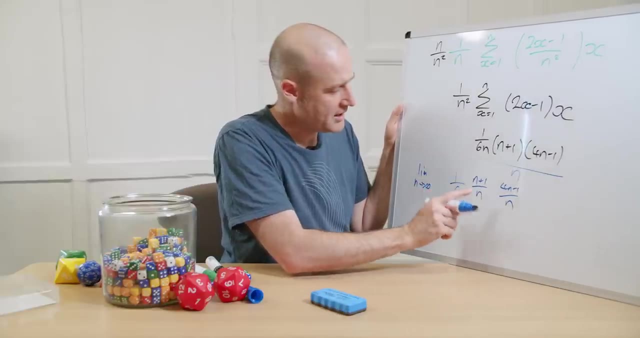 Like in theory, as we approach infinitely large n-sided dice. what would this ratio be? Well, if well, a six is a sixth. that's not changing n plus one over n, as n goes to infinity. that's just going to equal. that's going to equal. 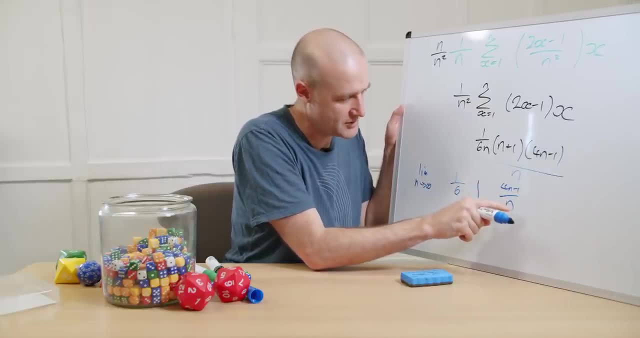 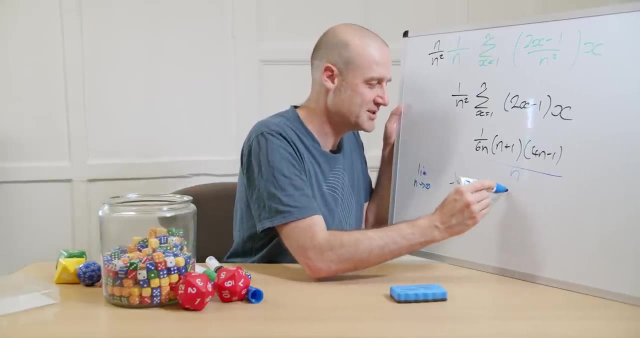 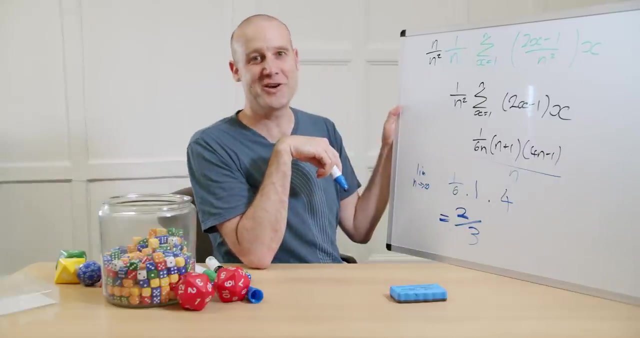 one, That's easy. put that in there, Right, Okay. And four n minus one over n, as n goes to infinity, that's just going to equal four. So actually it's one sixth times one times four. four on six, it equals exactly two thirds. 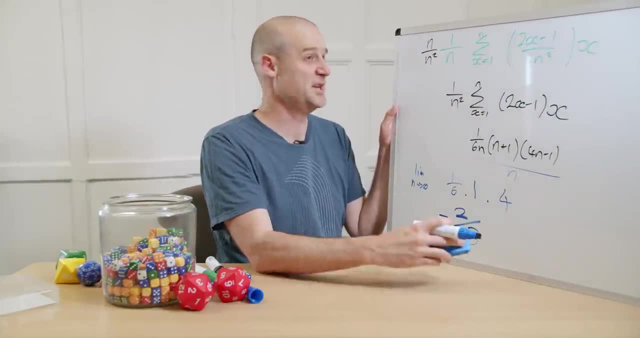 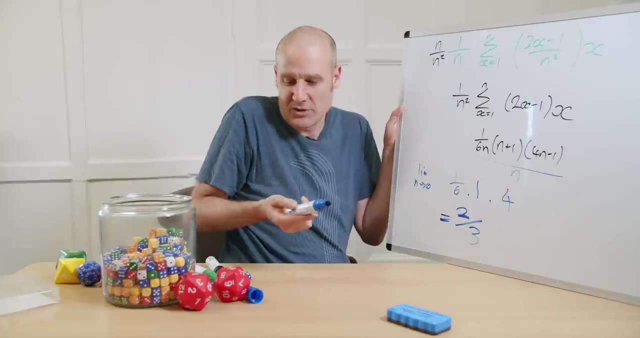 I couldn't believe it. So it's not two, It's probably something involving e. No, It's exactly two thirds. So there you are. So in general, just as a rule of thumb, if you're rolling two dice with advantage, the average result. 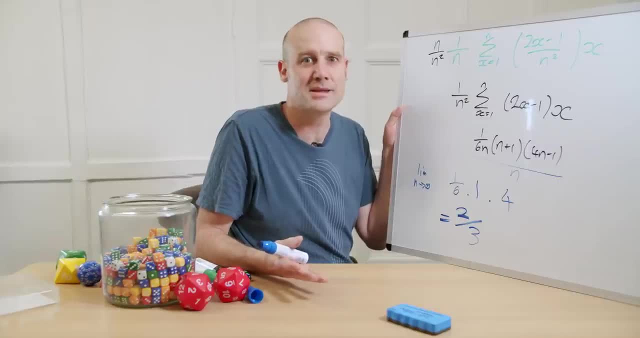 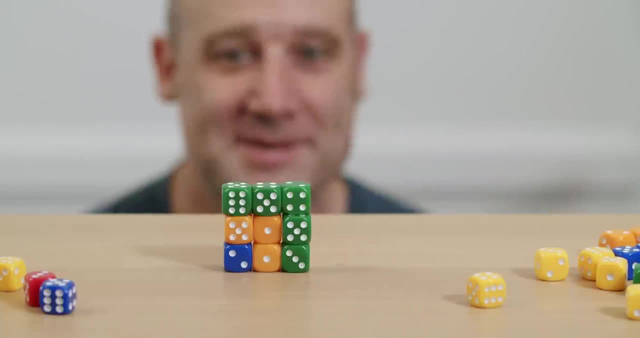 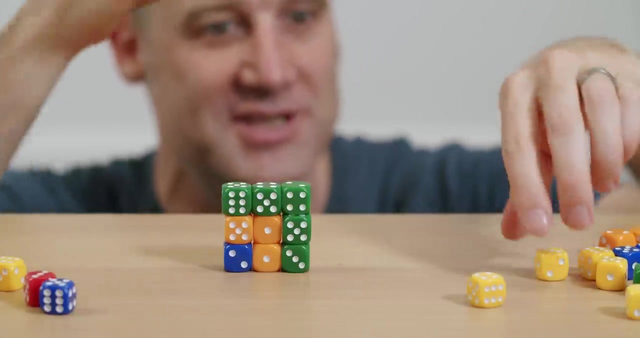 you're going to get is two thirds of whatever. the dice is Easy, But hang on. What if we were rolling three dice? Hey, Sound Up Maths Matt here. So I'm building a model of a diagram from before, out of dice. So it's now. 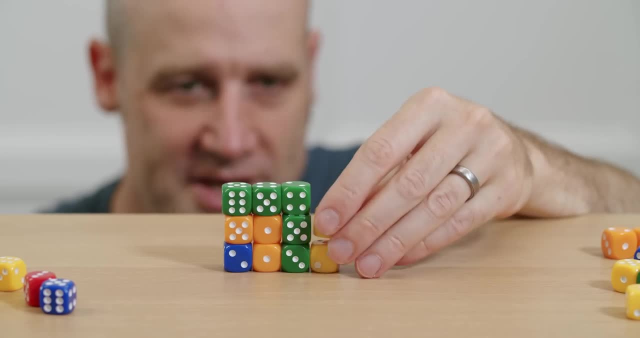 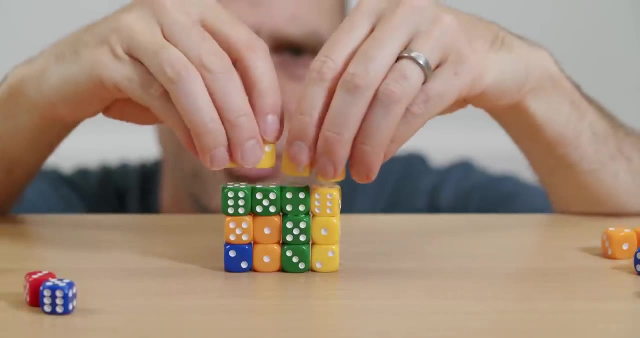 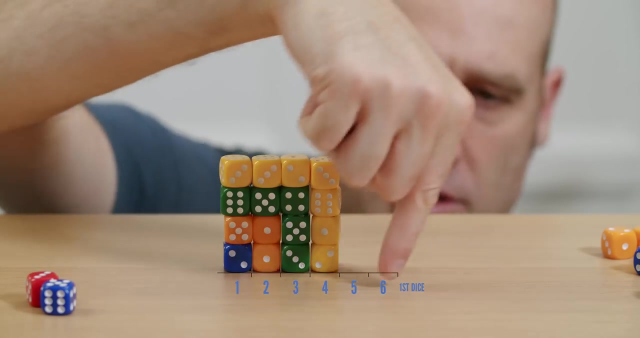 the dice chart made from dice, which is deeply pleasing, but it does mean you have to ignore the numbers. I'm just using these to represent the different regions, little areas in our two way sample space from before. So you've got what the first dice could be. 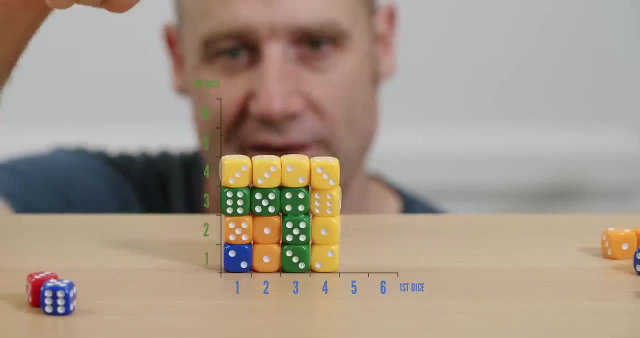 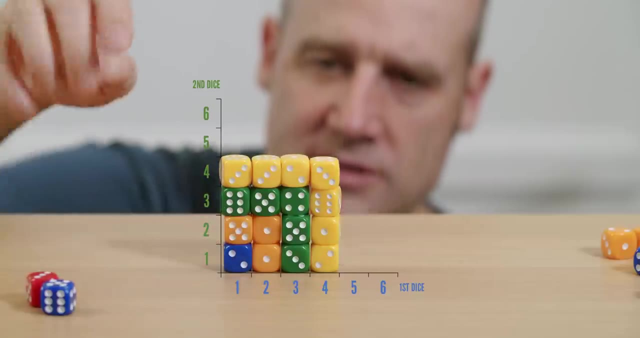 going across horizontally: one, two, three, four, and eventually I could build five and six. and now the orange ones. here are all the combinations where they're ones and twos, and so two's the biggest number, and then you've got where three's the biggest number. 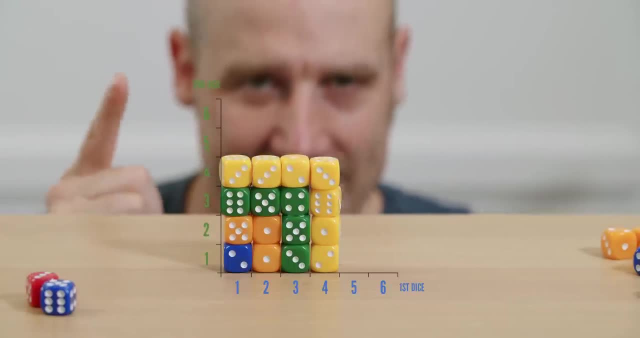 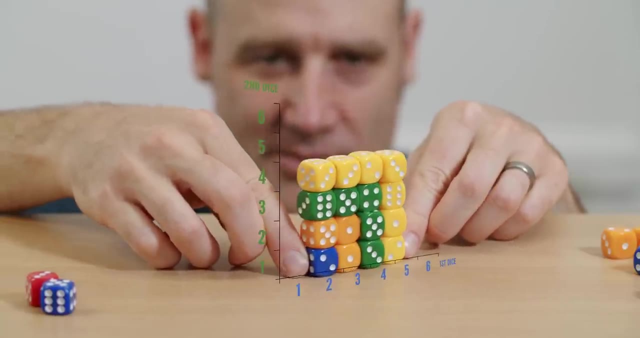 four's the biggest number, and I could build five and six. same as before. However, we now need to add a third dice. So instead of having a 2D plot with two axes, we're going to swing this sideways and have a third axis coming out. 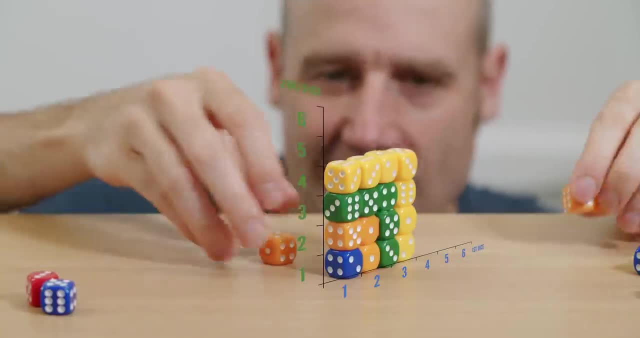 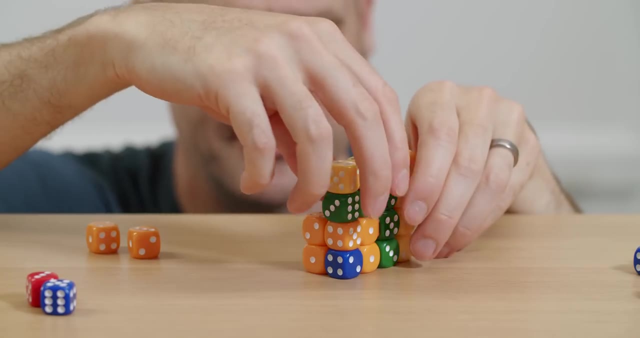 in this direction. We've got three perfectly good dimensions. let's use them so I can start building up this. here we go direction: oh, um, we need to put these. wait, I'm going to take these off for a second. oh, I should have glued these together. 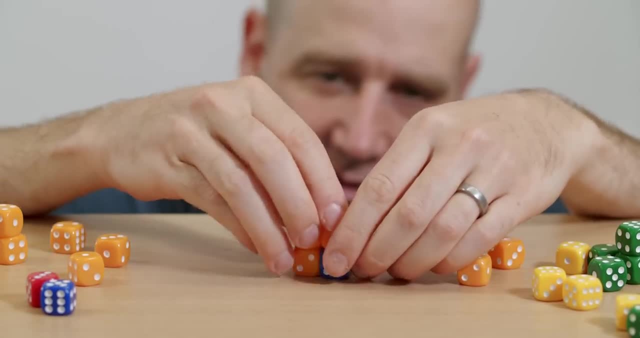 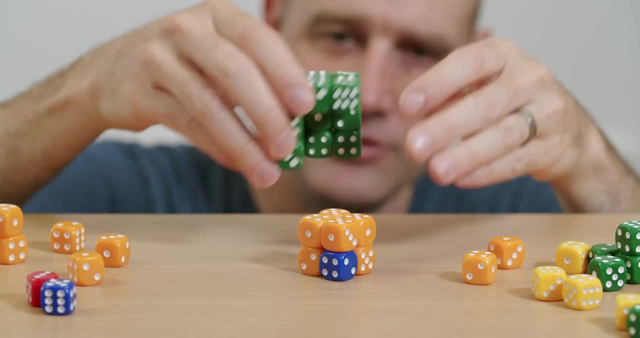 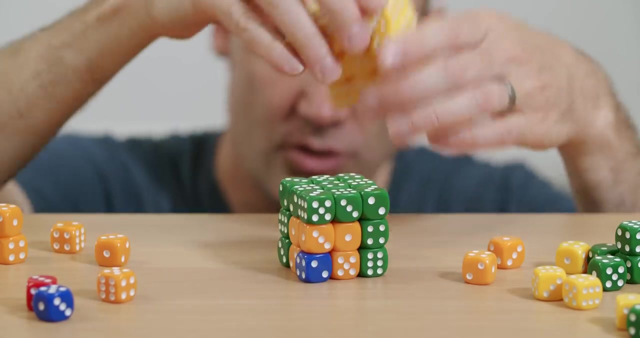 so I did there it is right. so there's the shell now of, in the 3D plot, all the combinations of the three D6's, which are ones and twos. we can then add on the shell for threes, because there's now one, two, three. 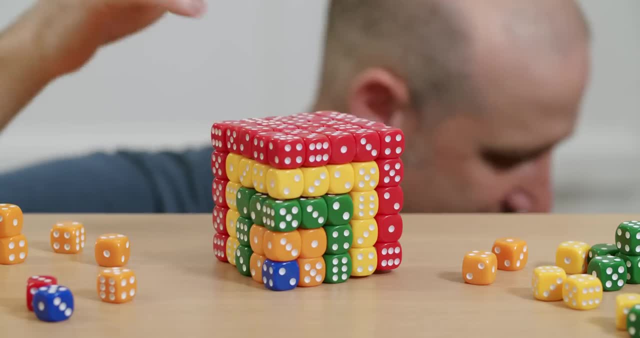 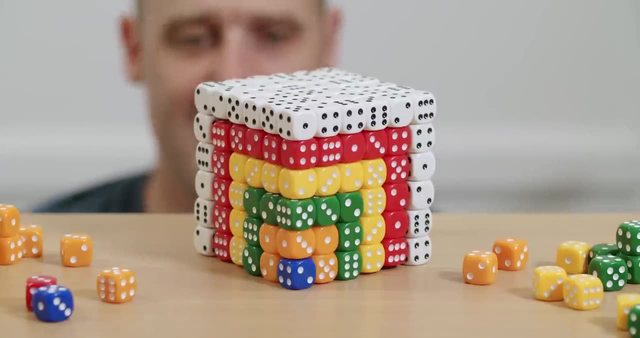 so these are all the dice, all the fives, finally, all the ones where six is the biggest value on the outer shell. and now you can see how much of an advantage rolling three and picking the highest is if you rolled a single D6 by itself. one and six. 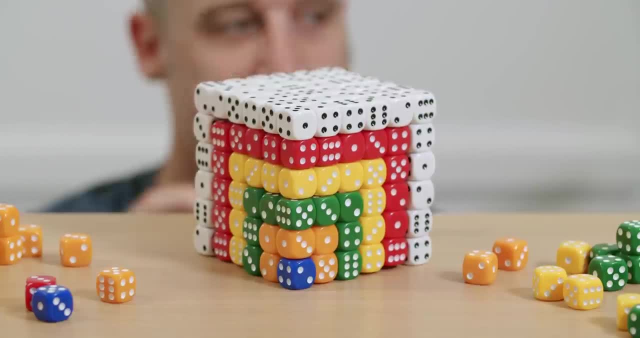 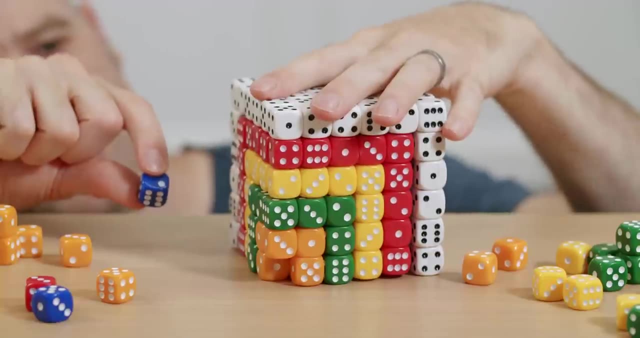 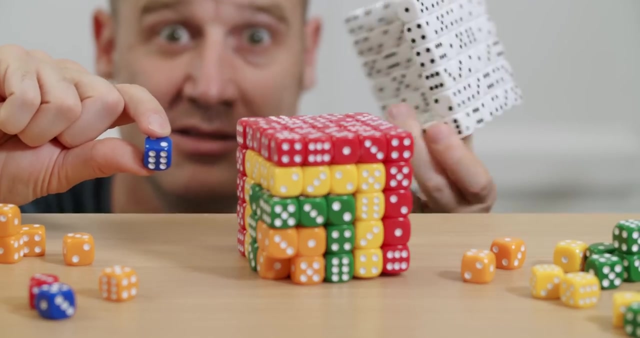 are equally likely if you roll three and pick the biggest. there's only one one of these out of uh 216 possible options where you get all ones and pick the biggest, and there's 91 cases where six is the biggest number. so, instead of being equal, 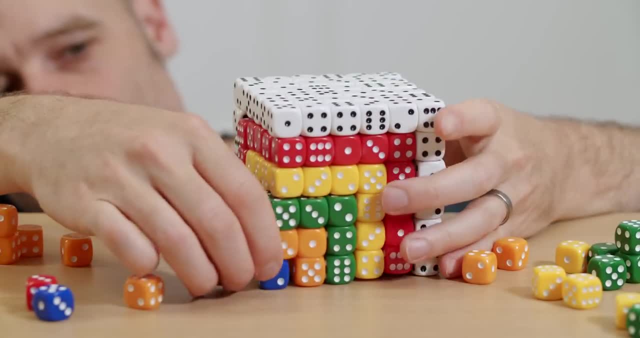 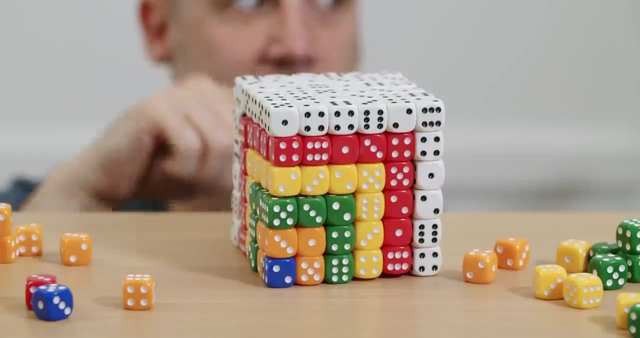 it's now one to 91, just ridiculous. and these aren't 2D areas anymore. they're not one over 36, which is the number of faces squared, they're one over the number of faces cubed, so they're one over 216. so each of these volumes. 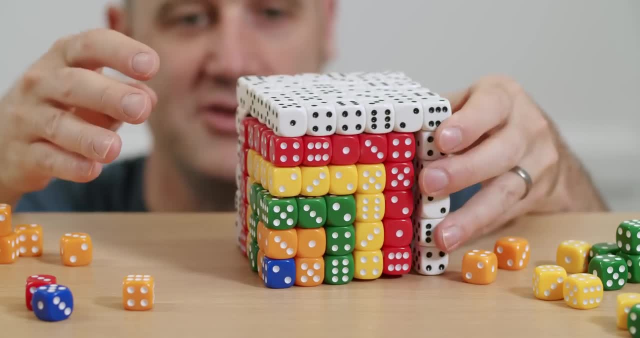 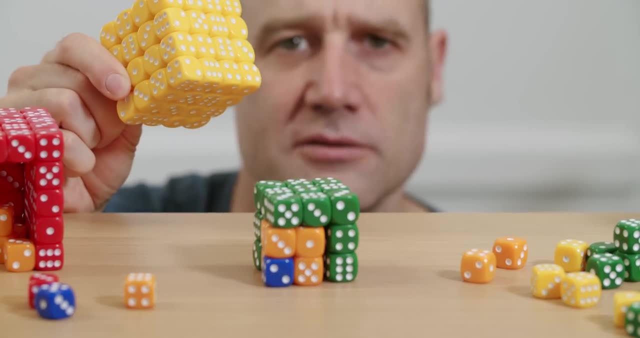 is a one over 216 chance of happening. there are 216 of them, and then you can work out each layer. but, unlike the odd numbers, there's no obvious formula for these values. i mean, they must have some kind of pattern, and they do. these are the centered. 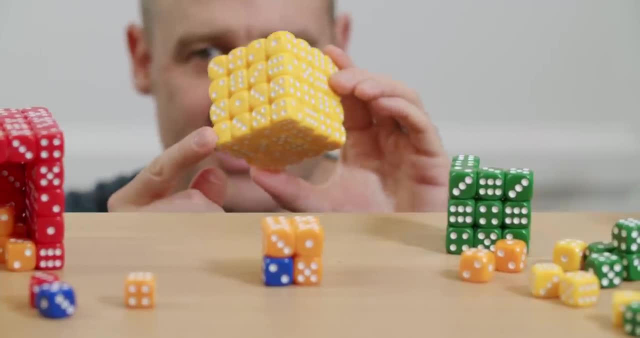 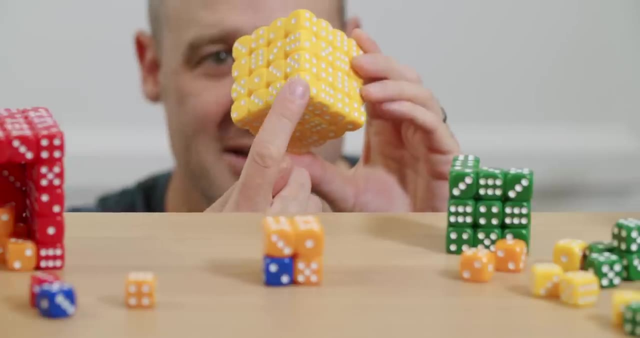 hexagonal numbers. so if i hold that one nice and still right in the middle and you get that focus, you've got one right in the center and then you've got concentric rings which are hexagonal numbers. so there's one and then six around it. 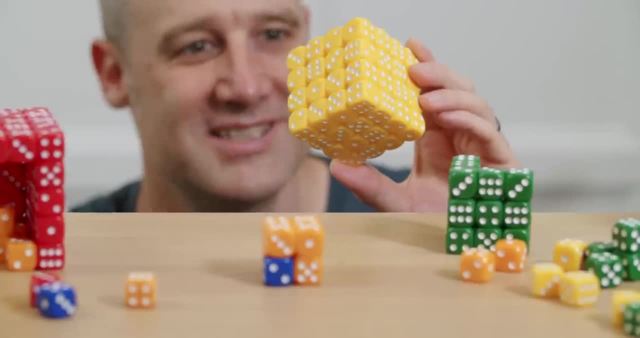 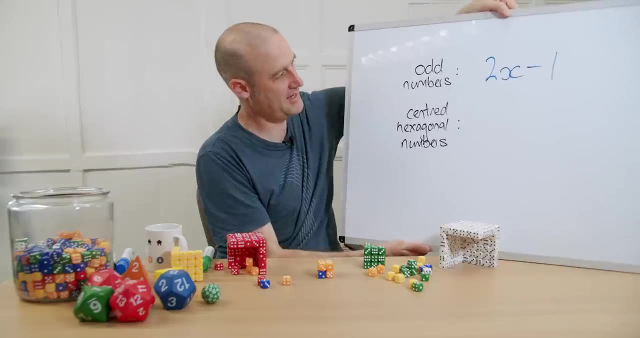 and then so on. it's so good and we can use that equation to do the working out. let's do it as soon as i get up. our equation for the odd numbers is easy enough. it's just 2x minus one and if you're unfamiliar, 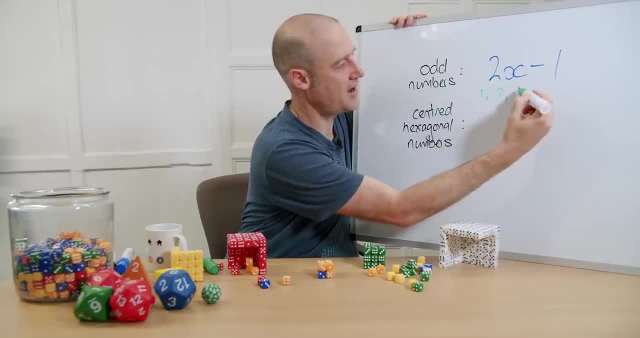 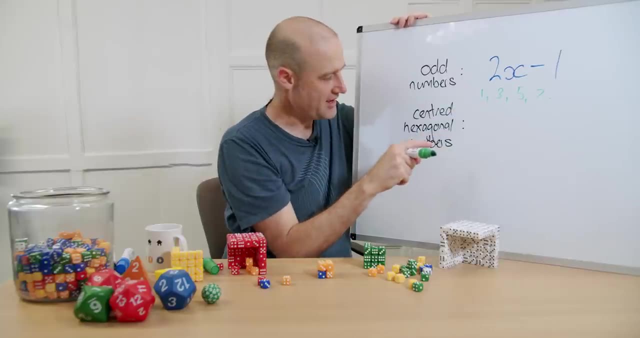 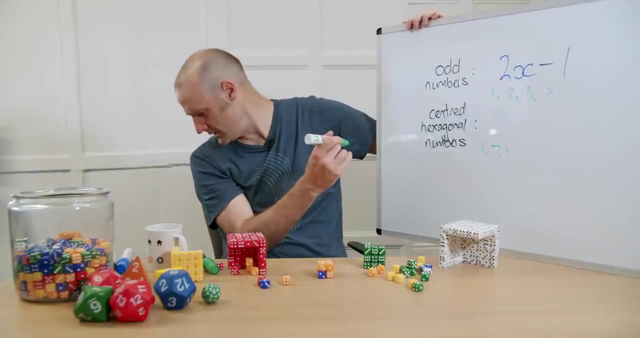 the odd numbers go one, three, five, seven and so on. and x is position one, gives you one. when x is two, position two, it gives you three. now the center hexagonal numbers: they go one, seven, pretty sure it's 19, and then down down there, 37. 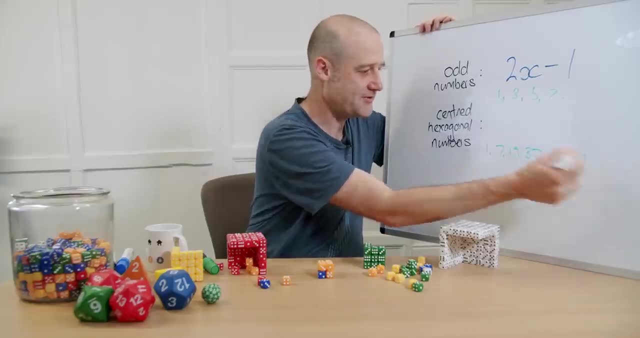 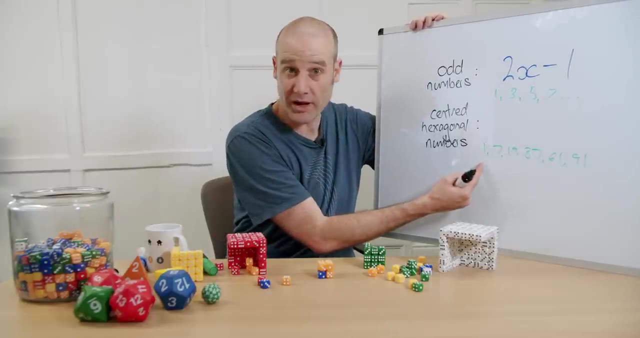 61, 91 and that 91. that was the final outer shell of this, and those are all the shells below. we need now some formula where you put it x is one and you get one. you put in x as two, you get seven, and that happens to be. 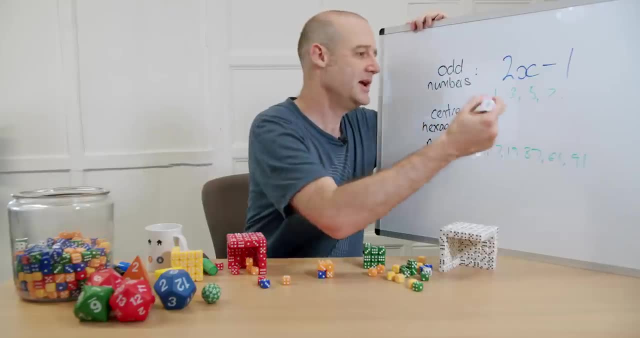 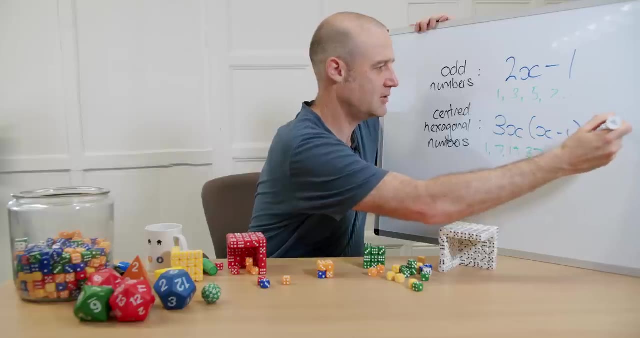 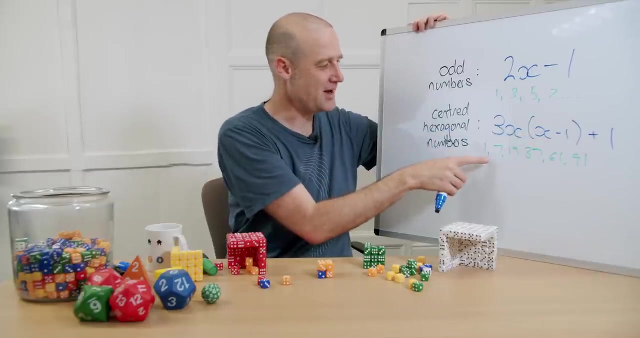 written it down as well. it's three actually. let's do this in blue so it matches: it is three times x outside of x plus one. you will occasionally see that with a plus where they've zero indexed this list, but i'm against my better judgment starting. 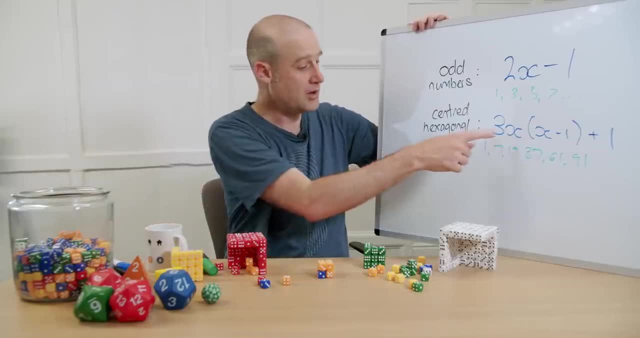 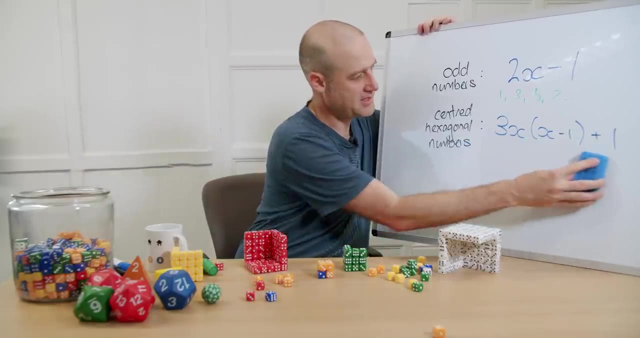 from one. so there's our formula for how big each shell is of all these different ones here. so now we can get rid of all this ridiculous extra bits and we're going to build that up into the equation for what the average value is when you roll. 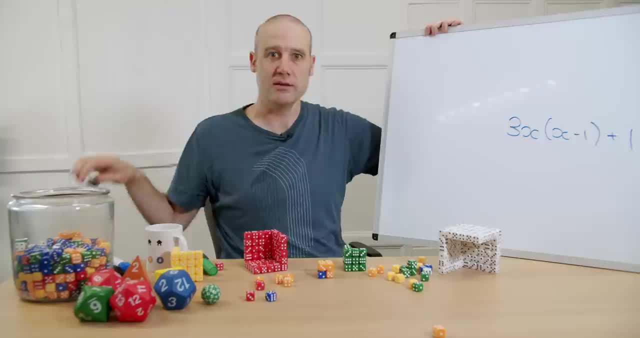 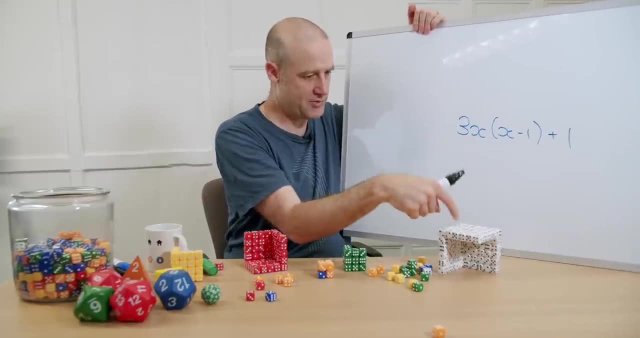 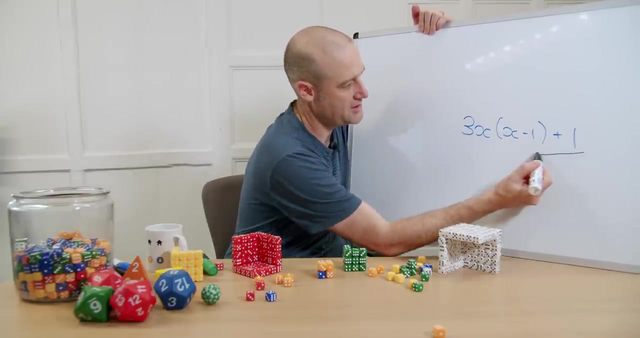 three dice and, with advantage, pick the biggest value. so first of all, that's the value of each shell. we need the probability of each shell, which is the number of cubes multiplied by the probability that each volume represents, which, as we established before, is just one over the number of faces. 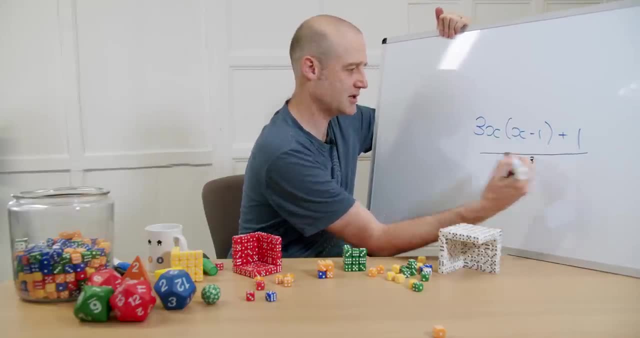 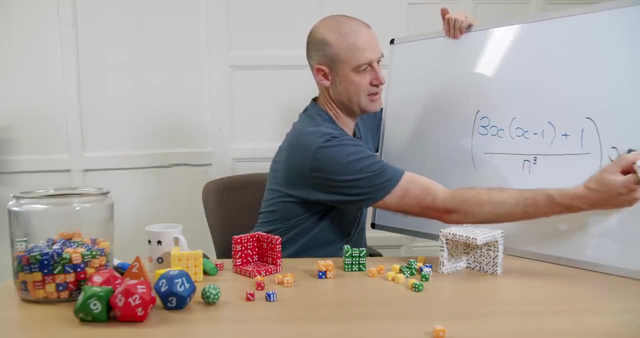 squared so we can chuck an- oh sorry cubed, chuck a cubed down there. that's the probability. we're now going to multiply that by the value which is the whole thing by each one is x, then we need to add them all up from the first face. 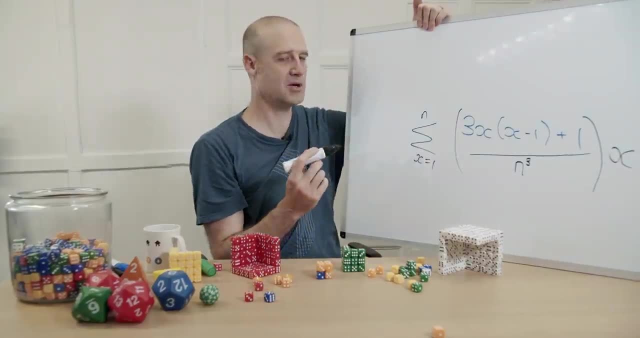 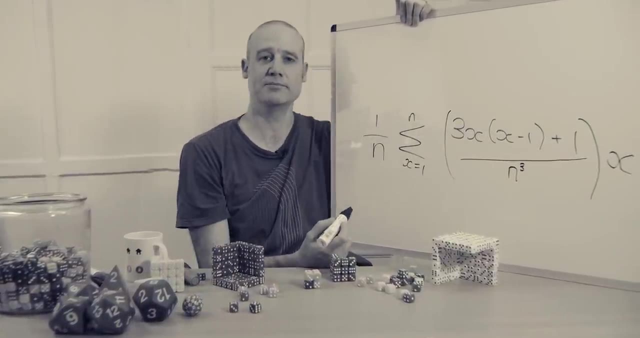 equi equals one up to the nth face future matt here to again clarify: past matt got a bit excited and put the one over n at the front, because that's when you want to compare the average value as a ratio to the number of sides. but then i decided 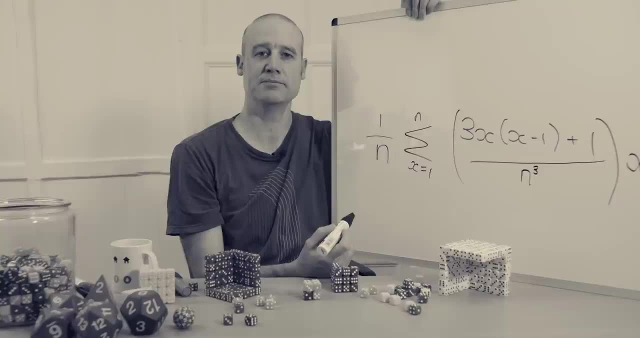 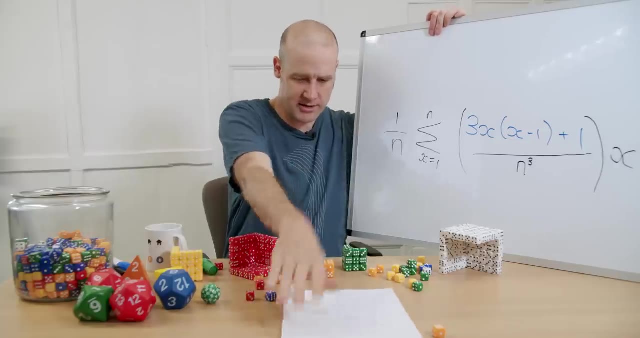 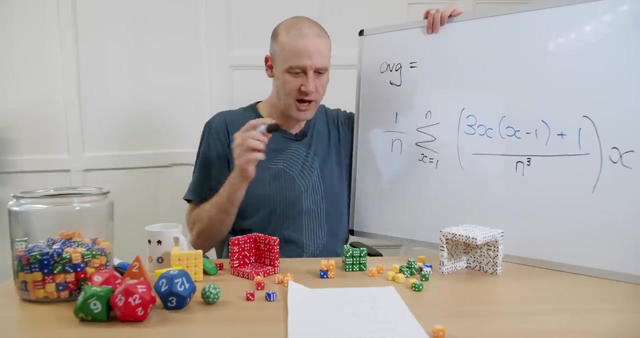 in hindsight. actually, i want to look at just the equation for the average first and then divide it by n to get the ratio- sorry, back to past matt- and i can give you the grand conclusion, the average value, if you roll three dice and just pick the highest. 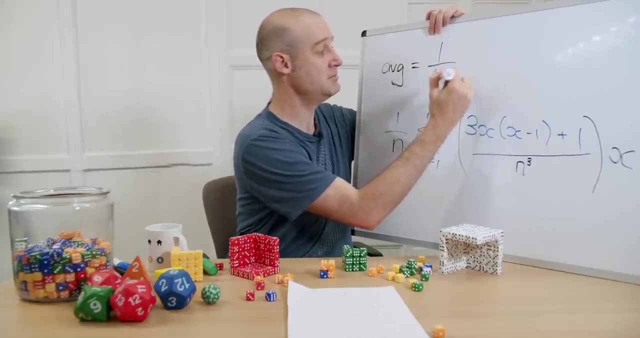 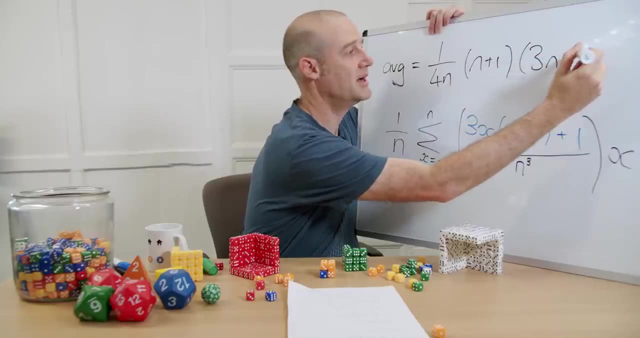 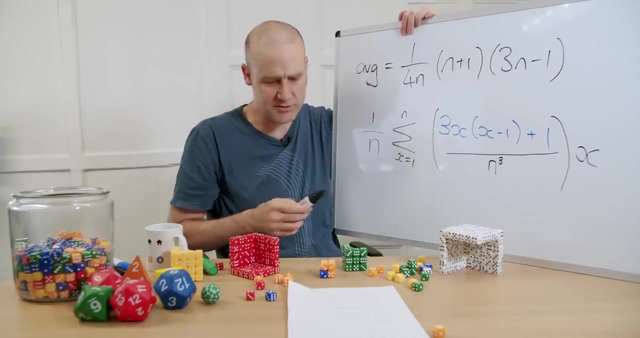 is one over this time four n pretty exciting times. n plus one times three, n minus one. nice and neat, check that out, and so we can go through and plug a bunch of values in. i did put in the value for a d20, so if your n. 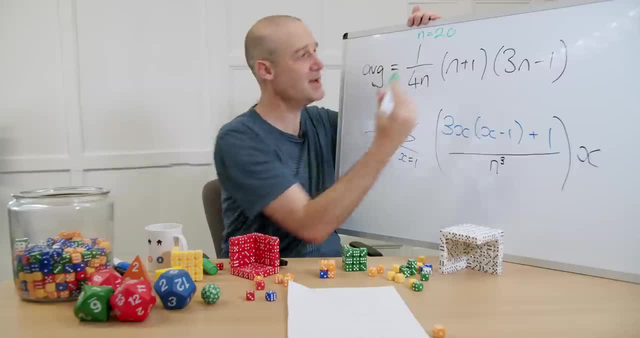 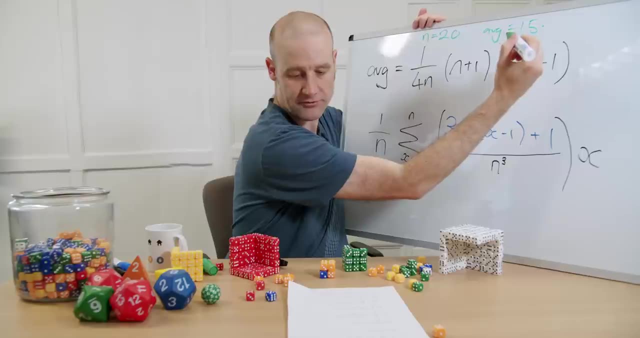 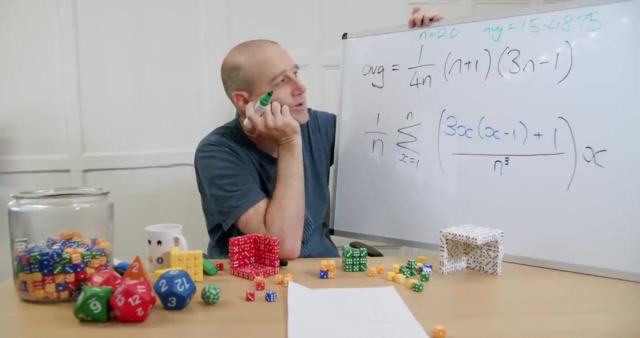 equals a 20 sided dice. you know your average value is for a d20 comes out at fifteen point. four, eight, seven, five. there we go. so just over three quarter. it's about three quarters. before it was two thirds. oh, that's too neat, too neat to not be true. 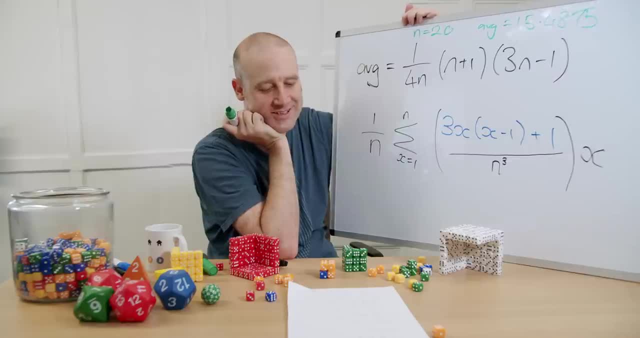 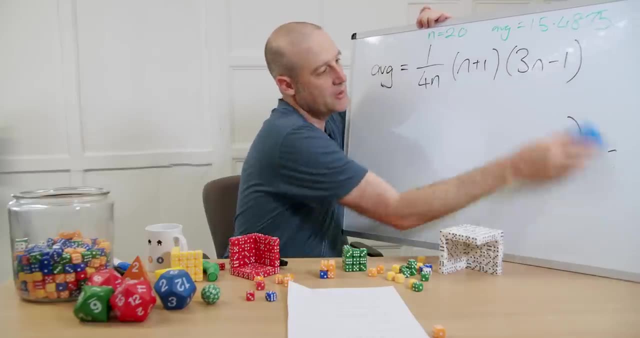 okay, let's find out. let's find out. so i'm going to get rid of our working out down here. oh, my goodness, we've now got at the top. there. that's our value for the average. we want to know now what the average is relative to n. 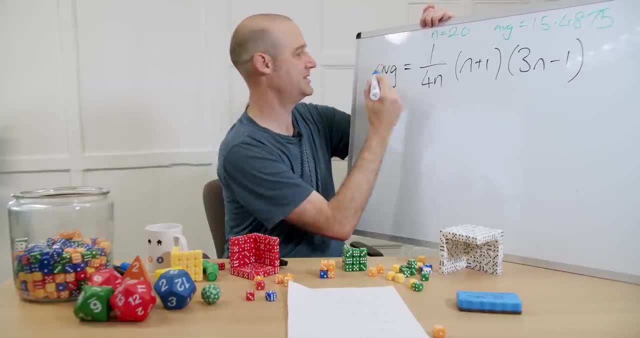 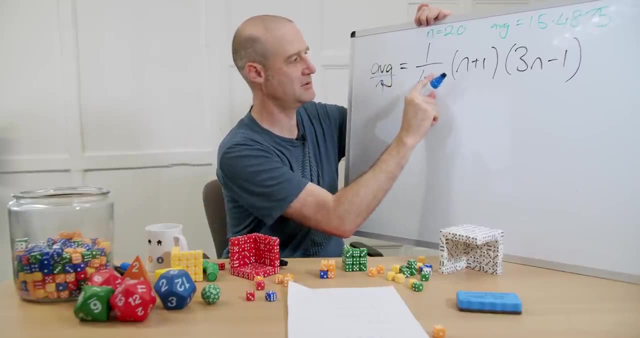 so we want to divide that by n again. so now this is the average on n. so we just put a squared down there and then, oh, actually that means we could rearrange it, we could take that n squared like we did before and we could chuck one. 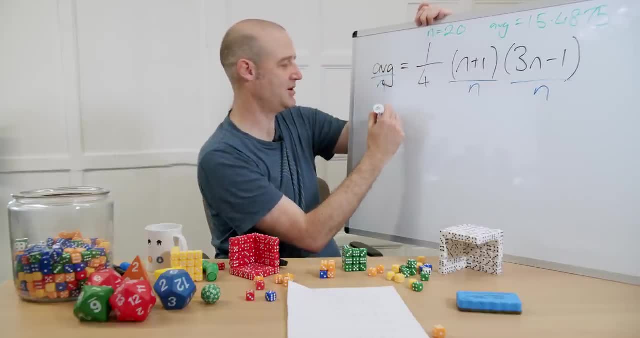 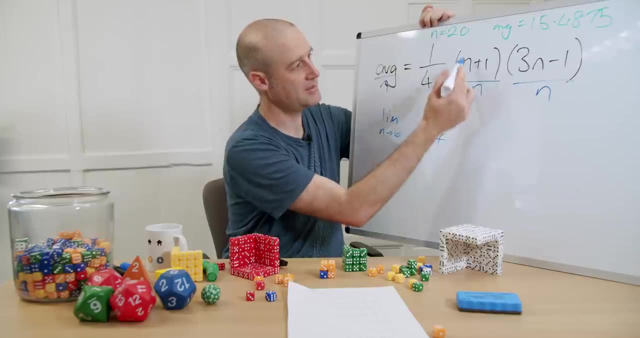 over there. we could chuck one over there. and now we want to know, as? what's the limit, as n goes to infinity, of this? well, it's going to be. the fourth is still going to be the same. that's going to be one, that's going to be. 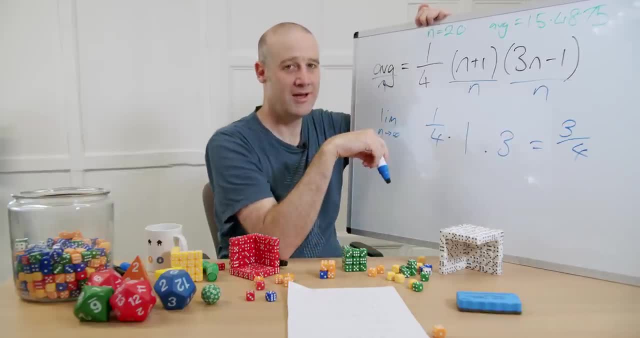 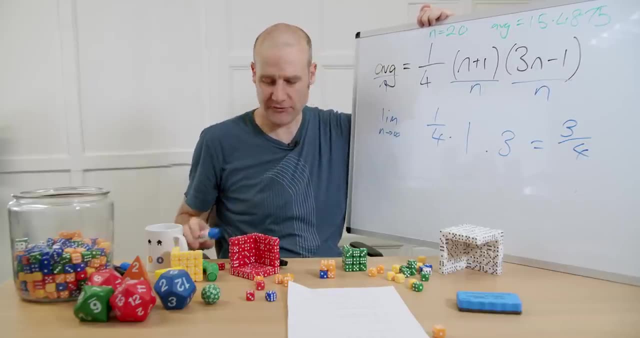 three, it is. it's three quarters. there you are okay. so turns out, if you roll two dice and pick, the highest is two thirds if you roll, and just for comparison i'm going to put that over there. so when we had two dice, the- oh, no wait. 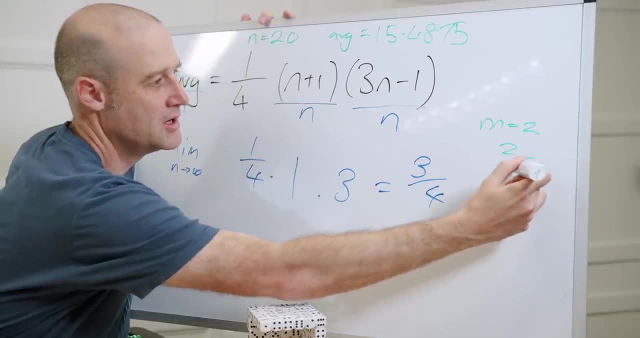 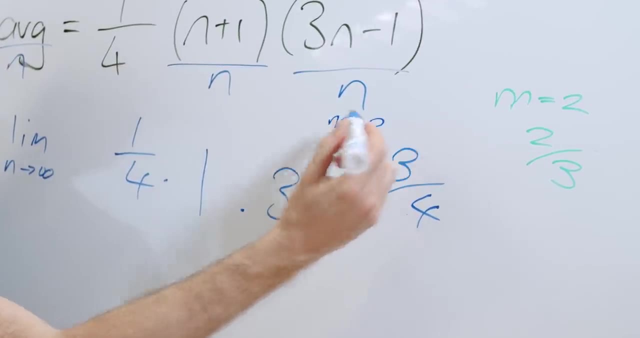 m if we had m dice, so we had two dice case. that was two thirds. this here. this is our three dice. this is the m equals three dice case. this is three quarters. the big question now on everyone's lips is if we worked out the m equals. 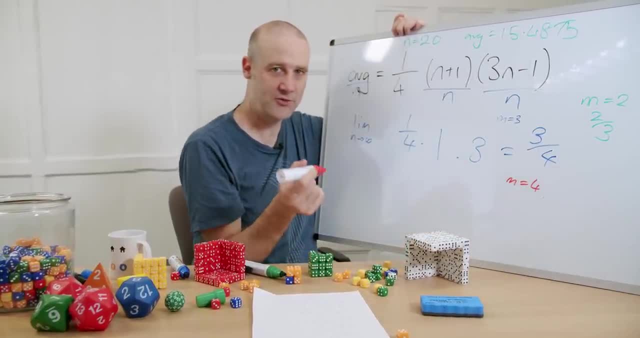 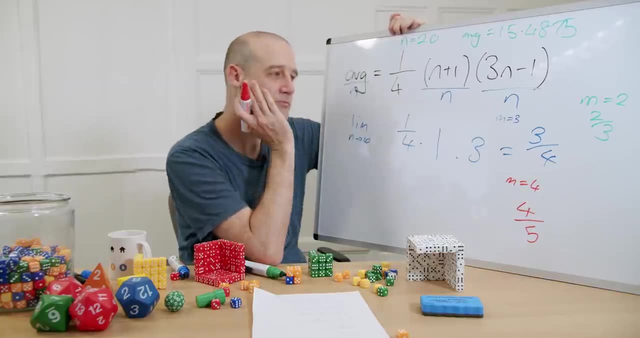 four. case you roll four dice, you pick the highest, will the pattern continue? will it be four fifths? there's only one way to find out, and it involves hypercubes. right, if we're rolling four dice at once, we're going to need four orthogonal directions. 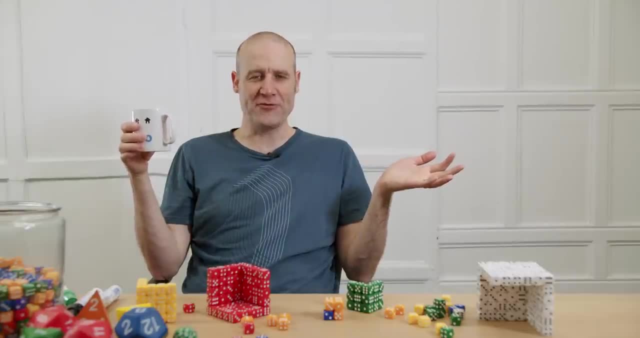 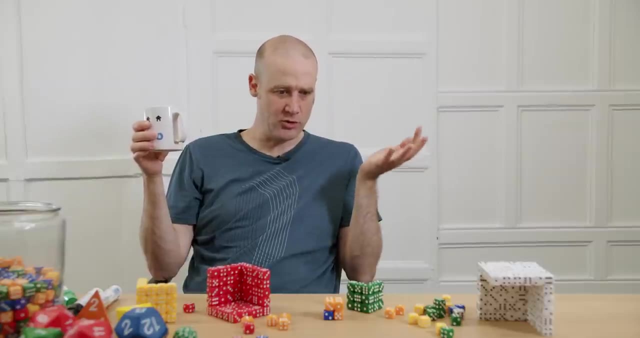 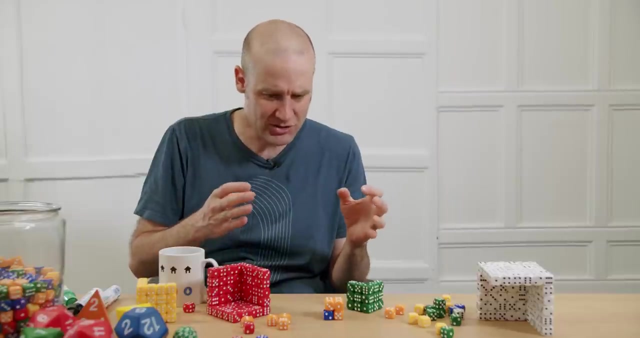 on our right, right, right, right, right, ah, space of all possible results, which means we're going to need more dice, more glue and more dimensions- and i'm not going to start gluing together, as tempting as it is, hypercubes, but in theory, each time you add. 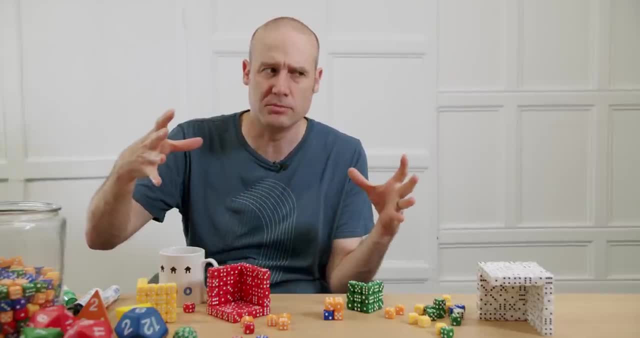 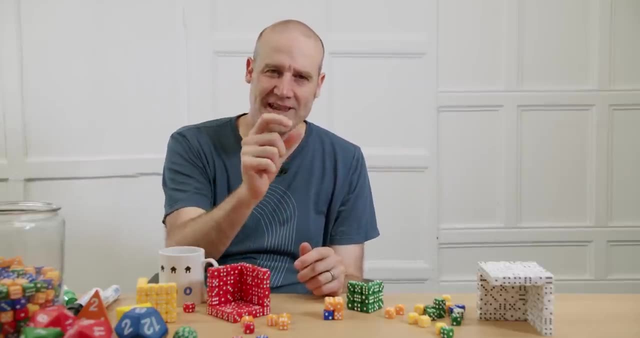 another number on the dice. you just it's a bigger and bigger hypercube of possibilities. you have to work out the four dimensional shells, how many 4d content like hypervolumes there are in, uh, and you know what? we're just going to work it out. 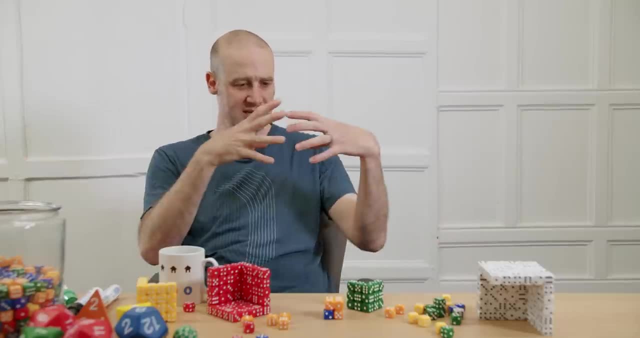 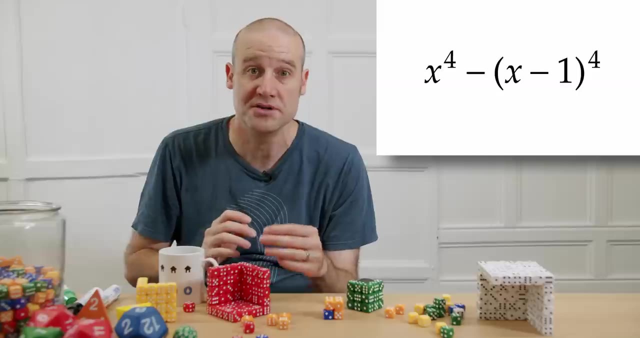 using algebra, know what the equation is for each of these, like each of the shells in four dimensions, because it's just the difference between two consecutive hypercubes. it's x to the four, subtract x minus one to the four and spoiler. we could have done that um with all the other ones. 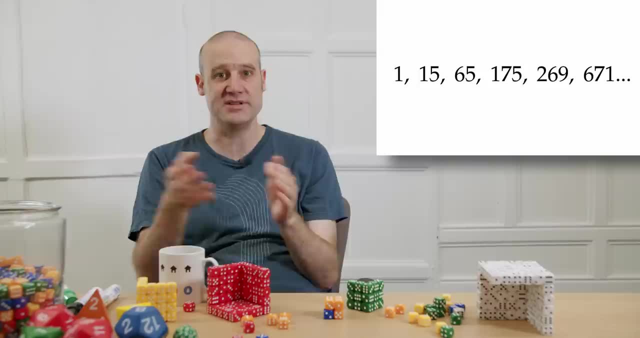 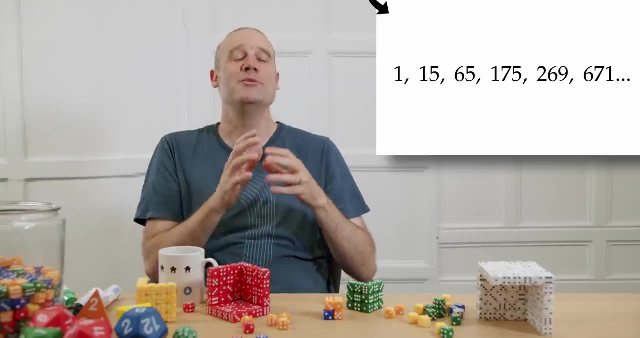 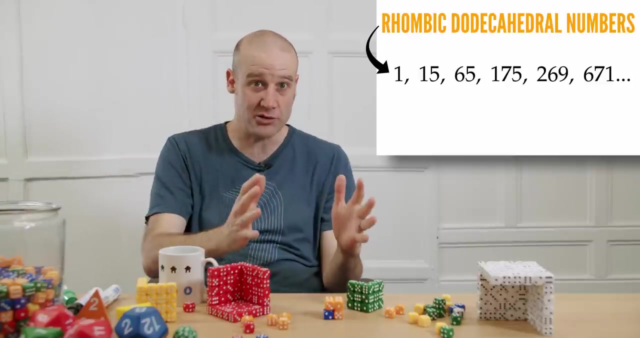 anyway, the point is we've now got this sequence of numbers that goes 1, 15, 65, 175, 269, and what's the pattern? well, these are the rhombic dodecahedral numbers. so we went from the odd numbers to the hexagonal numbers to now this is the rhombic dodecahedron, the greatest of all the dodecahedra. 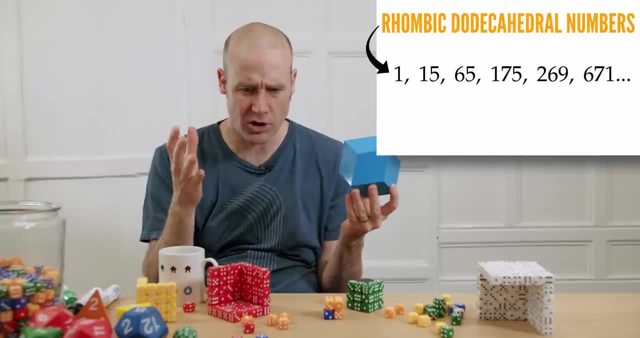 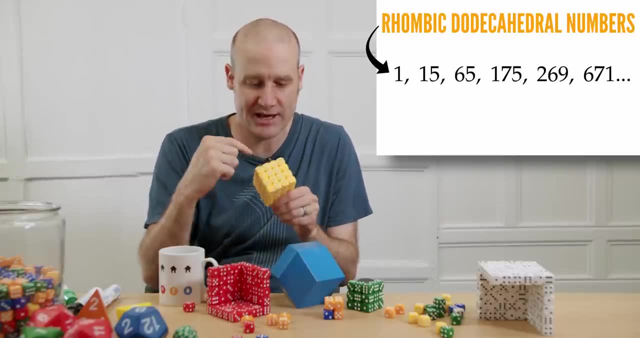 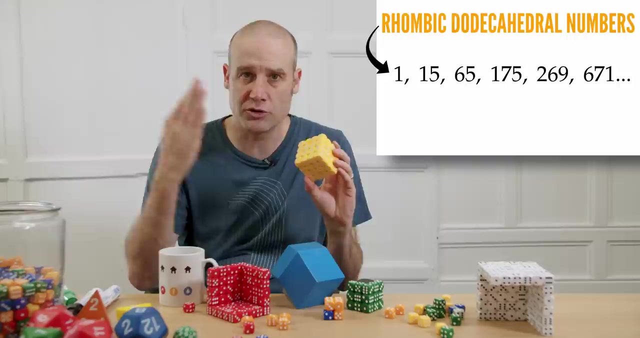 and that actually makes sense, because if you've got a square, the, the diagonal cross section, like the center cross section of a square, is a line, and actually that's why, when you look at it from the corner, you see a line, but it's wrapped around and the middle cross section of a cube is a hexagon, which 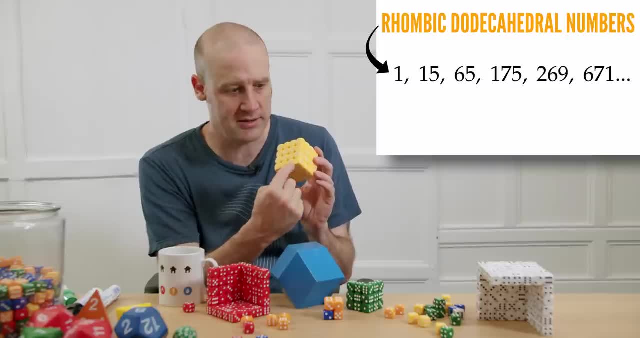 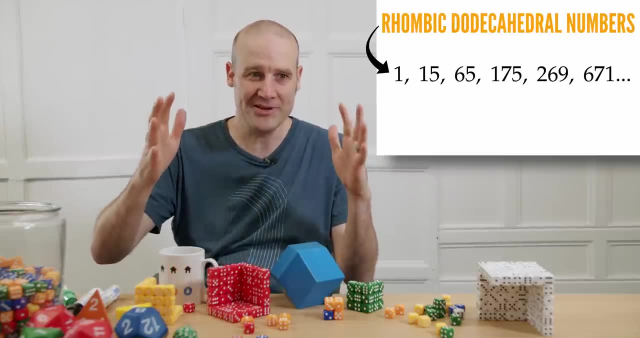 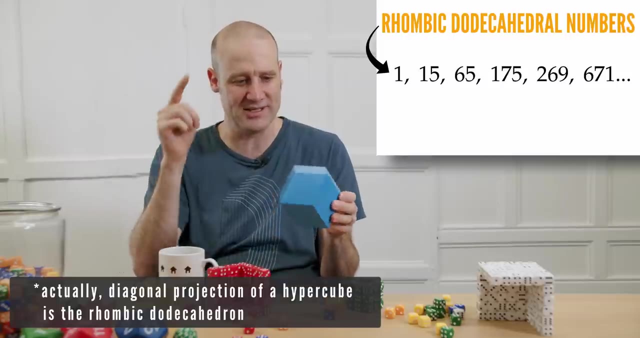 is why, if you look at it perfectly, corner on, it looks like a hexagon and they're centered hexagonal numbers and, as some of you may know, if you get a 4d cube and you cut it perfectly in half on the on the hyper diagonal, the cross section of the 4d cube is a 3d rhombic dodecahedron. it's so pleasing. 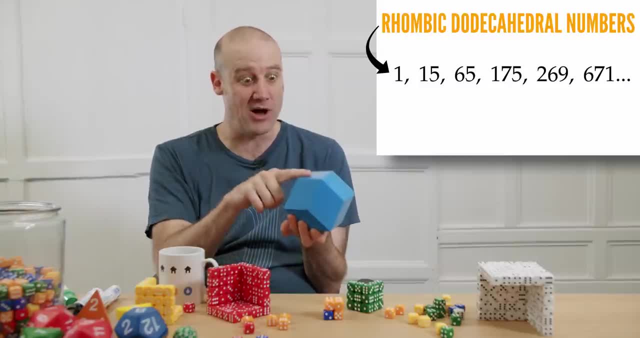 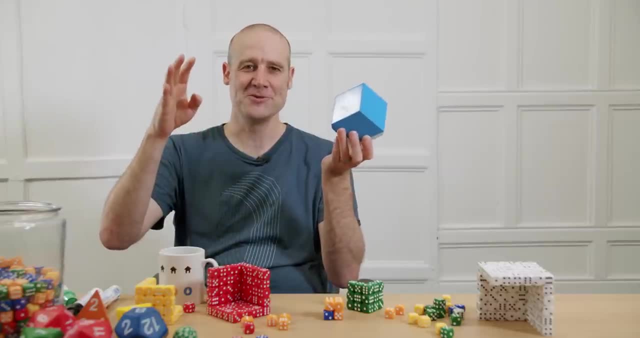 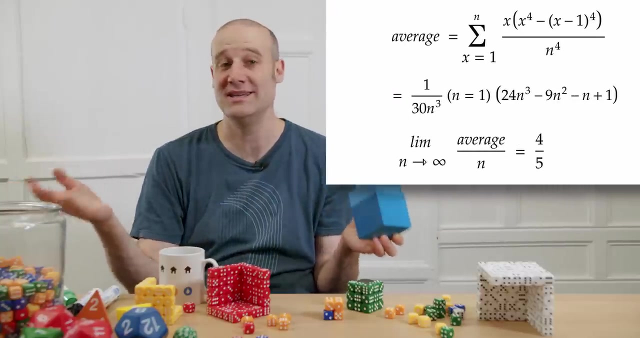 think of it like the 3d hexagon and- and that's why, the numbers: if you add together consecutive, centered, rhombic dodecahedron numbers, you get the hypercube numbers. ah, maths. the point is we've got the equation, we can crunch it through it like we did before. indeed, i've done it. give it a go, it's good fun and it. 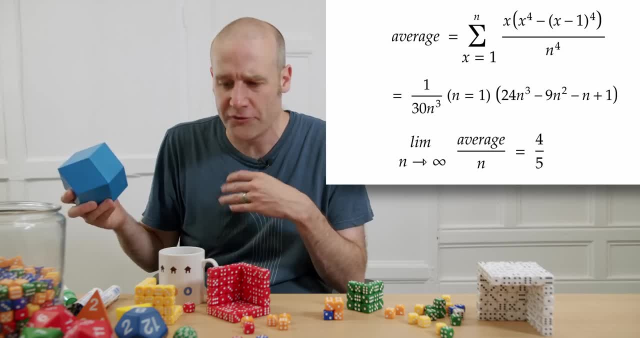 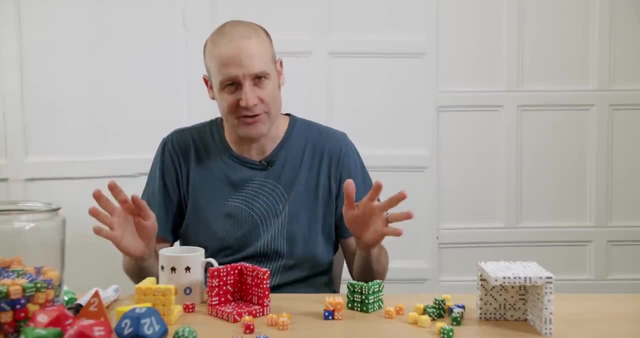 ends up four fifths, it's four fifths. if you roll four, you don't have to worry about the hypercubes and the rhombic dodecahedra, all that jazz. if you roll four dice and pick the highest, you will get, on average, four fifths of whatever the value of the dice is. 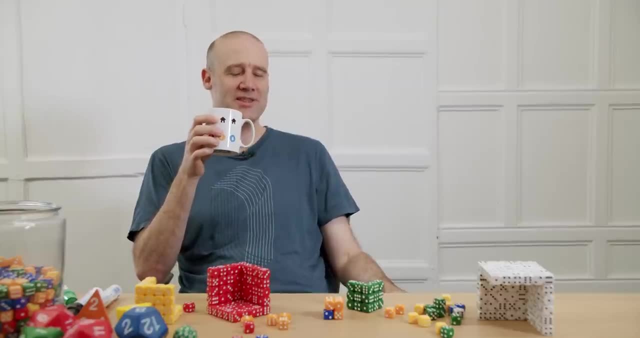 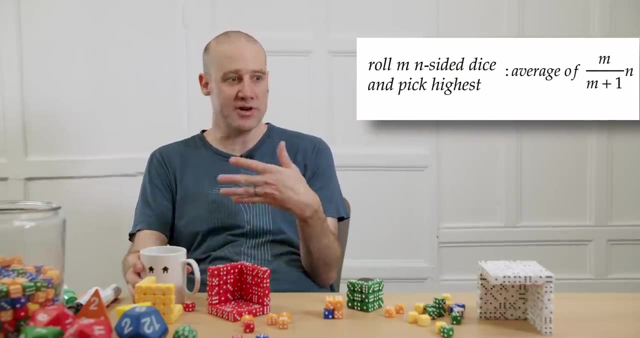 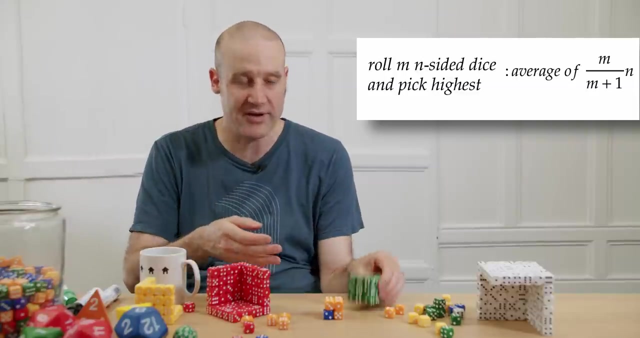 sort of some of you have already thought- does this work in the opposite direction? so it seems very, very likely that if you roll m dice you end up on average- if you just take the highest one- getting m divided by m plus one times however many faces you've got that seems. 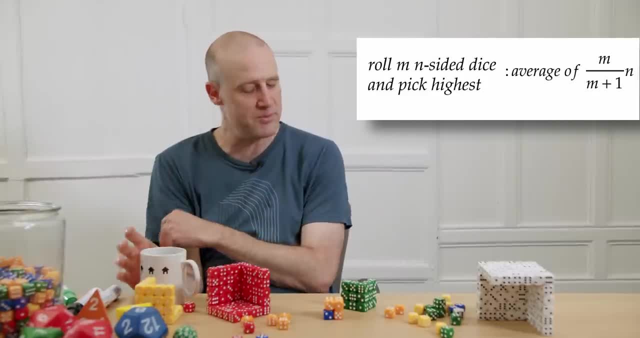 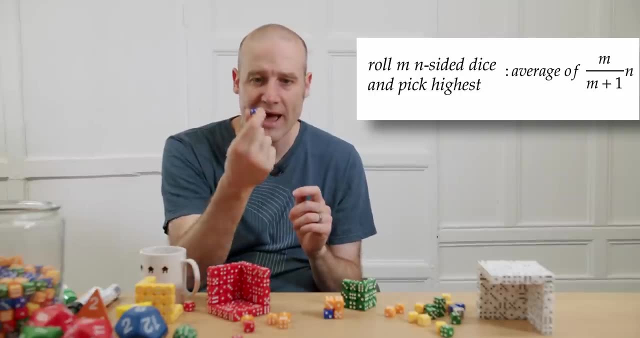 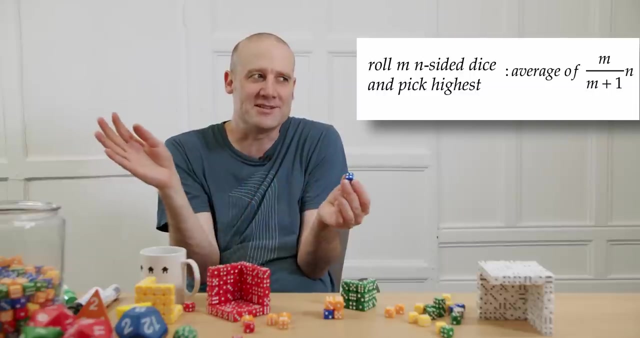 very, very likely, and we haven't proved that- carries on going up. pretty sure it does. if you go backwards, you put in the case for one dice a single one m. it should be half. it's not half. it's well, it would be it is in the case of if there are infinitely many faces, as it tends to. 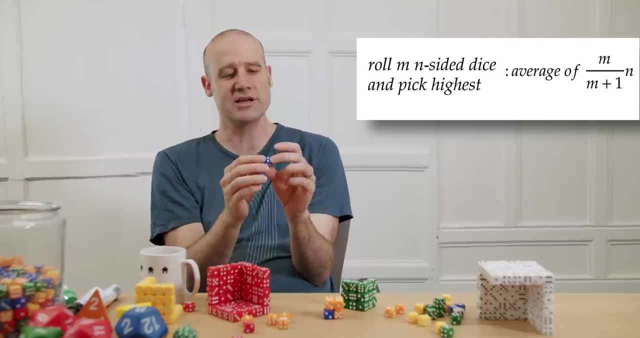 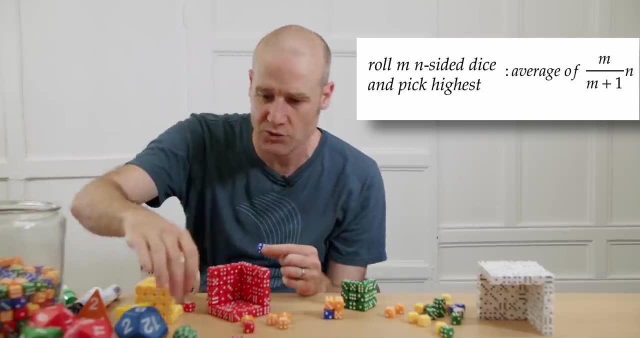 infinity, which is how we're working out. it's exactly half. but it's not exactly half, it's a half of the value. so the average volt roll on a d6 is three and a half. the average roll on a d- i'm d20, here we go. it's ten and a half on my d60.. 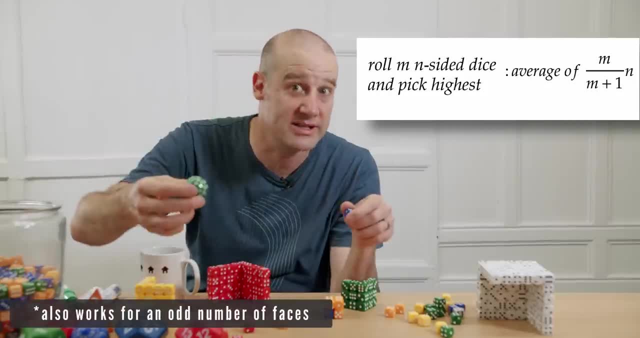 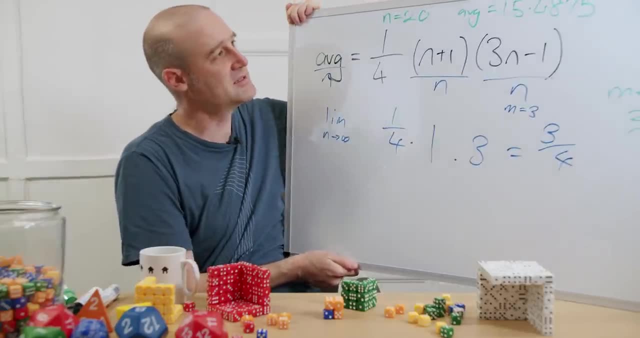 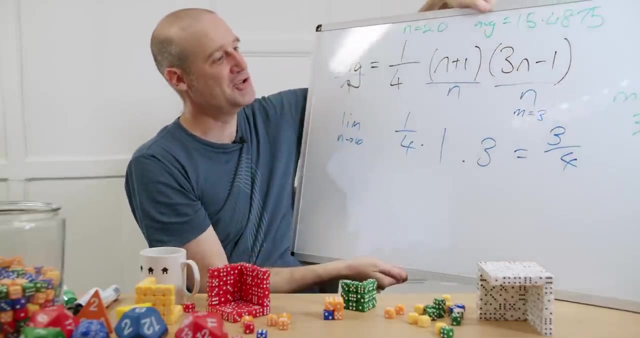 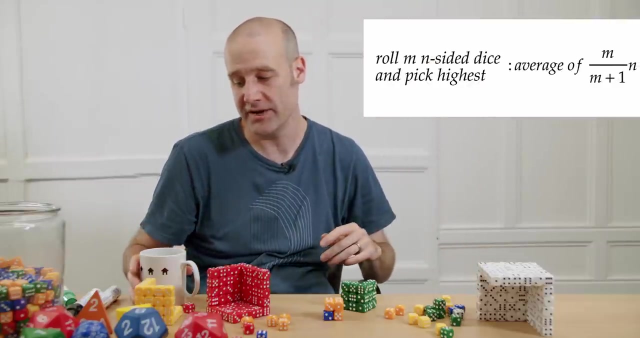 half, because there's an even number of faces and you're always getting a whole number and in fact before, when we worked out the average for rolling three d20s, 15, which is three quarters and a half. so i my conjecture is: it's always for m dice rolled with advantage. it's m divided by m plus. 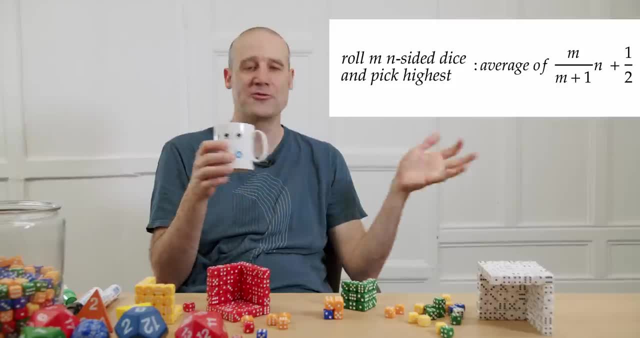 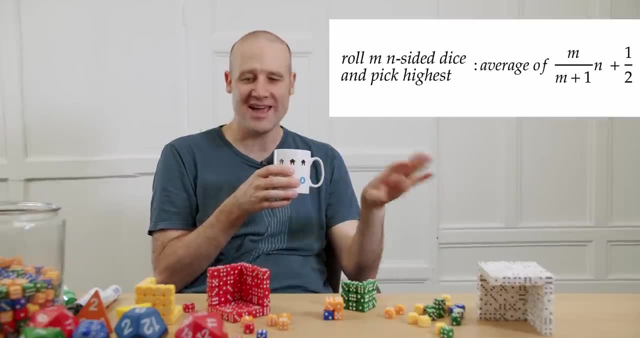 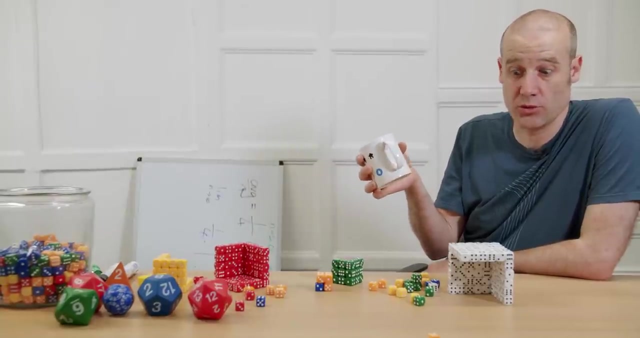 one times n plus a half. feel free to prove, disprove or extend my conjecture. i think it's good enough for the size and number of rolls in a standard dnd game. so there you are, if anyone ever says there's no practical reason why you want. 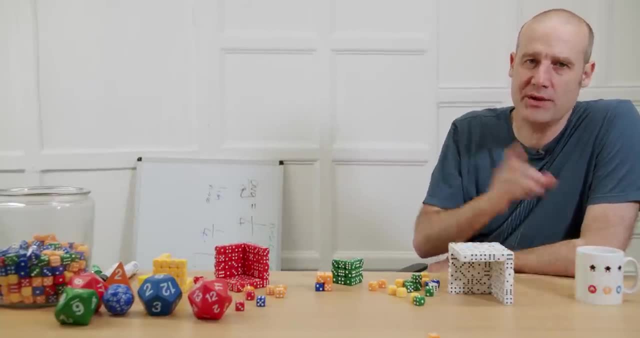 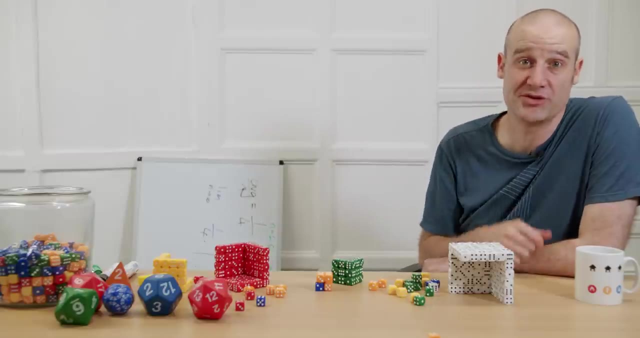 to know that the central cross section of a 4d hypercube is a 3d rhombic to decahedron. now you can just throw some dice in their face: super applied mathematics. so anyway, thank you so much for watching this video and thanks to jane street, who not only sponsor this video and my channel. 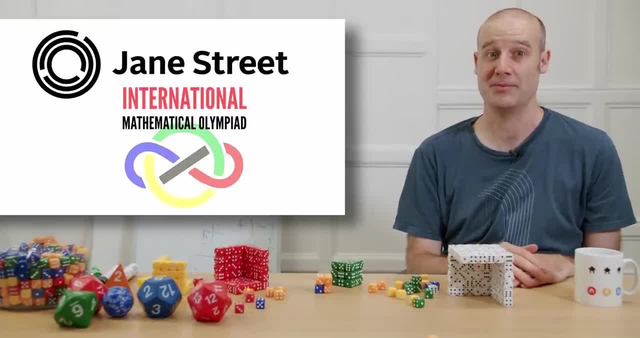 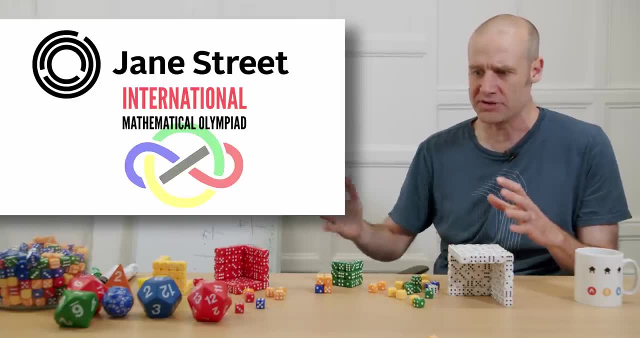 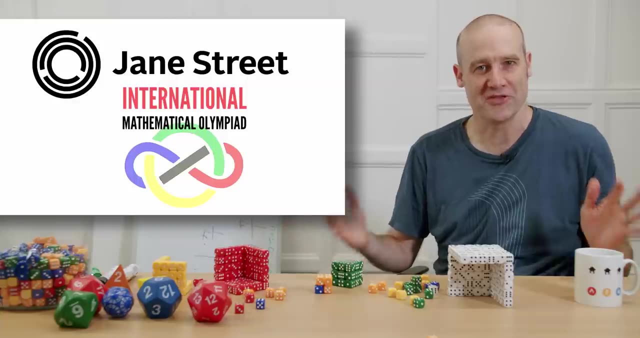 they also sponsor the international mathematical olympiad which is happening this year from the 6th to 16th of july in oslo, norway, and it's where teams all around the world send six pre-university math students to compete in like. it's like the mass version of the hunger games. it's like the number games they all have to run.